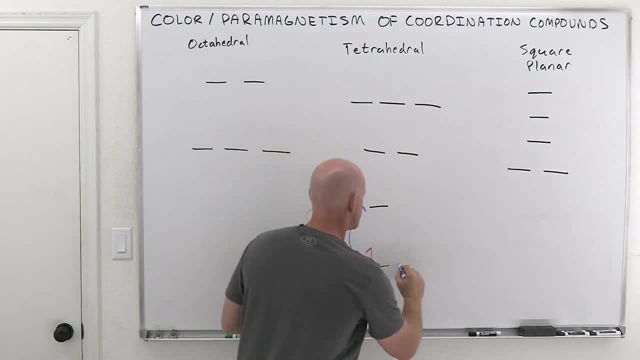 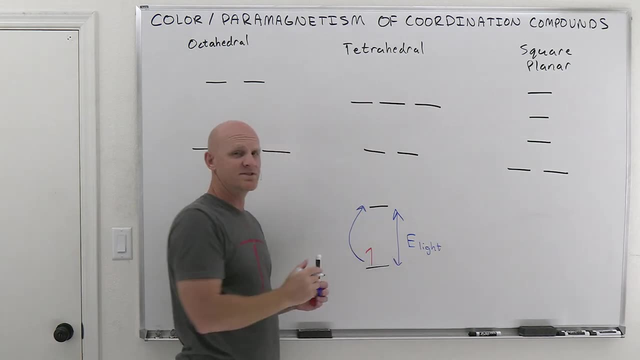 orbital to this higher energy orbital. Well, it turns out that the energy of that light is going to correspond perfectly to this gap in energy between these two orbitals. Well, if you take a look at, say, the oxygen in this room, well, the oxygen in this room, 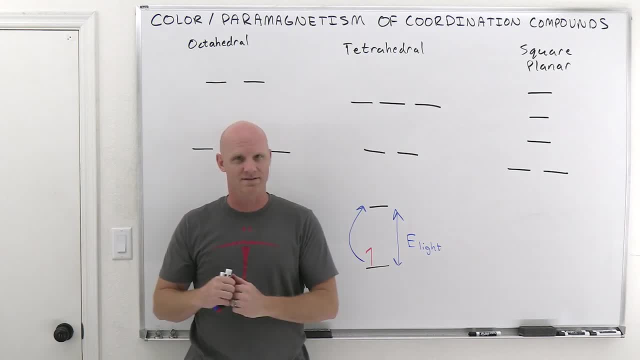 I say, take a look at it, but it's invisible. and it's invisible for a reason. If you look at the highest energy orbital that has electrons and oxygen and then the lowest energy orbital above that, the gap is huge. and it's so huge that the energy difference corresponds to the energy of 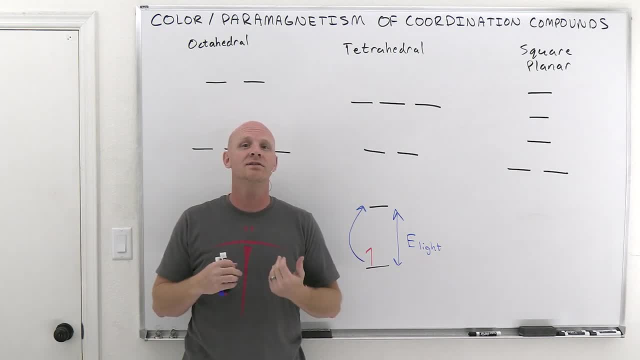 ultraviolet light which your eyes and my eyes cannot see, which is why we can't see oxygen in this case. So if a compound is going to appear colored, then it needs to absorb light that you and I can see, and that's colored light, visible light. It needs to absorb light in the 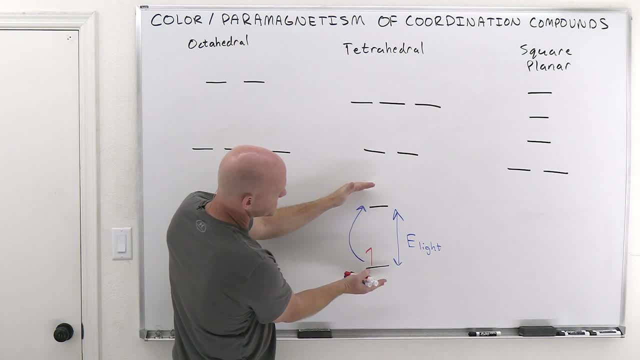 visible spectrum and unfortunately again, this gap compared to oxygen is going to have to come down in a significant way. That gap is just too big in, say, oxygen and things of this sort. Well, it turns out, comparatively speaking, then, if you take a look at the gaps in energy, 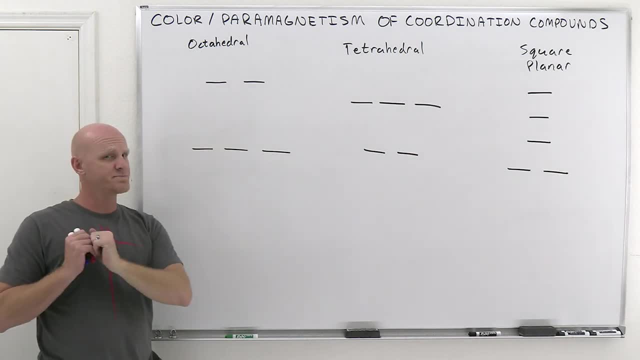 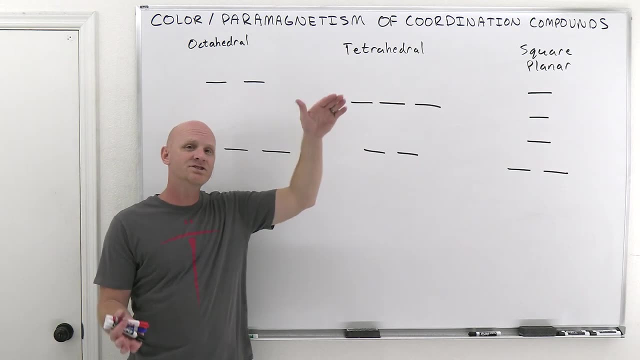 in the d-orbital splitting, whether that be in an octahedral complex, whether it be low spin or high spin, in a tetrahedral complex, or in a square plane or complex. if you look at some of these d-orbital splittings, that energy gap is much smaller than the one I just referenced in. 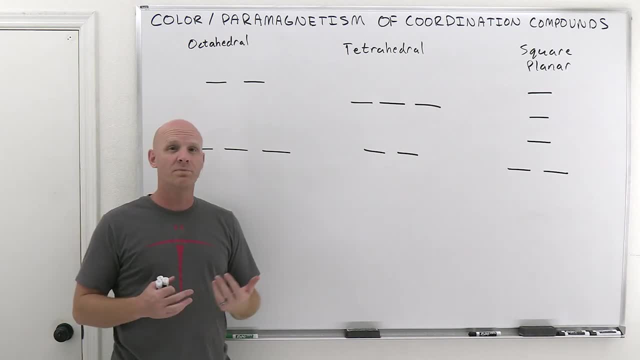 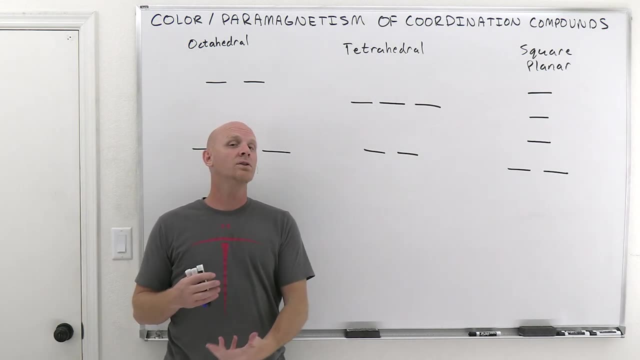 say oxygen or something like this, and as a result, it often corresponds to visible light, and so visible light might get absorbed. Now, one thing you have to realize, though, is that even even though a certain color of visible light is going to get maximally absorbed, 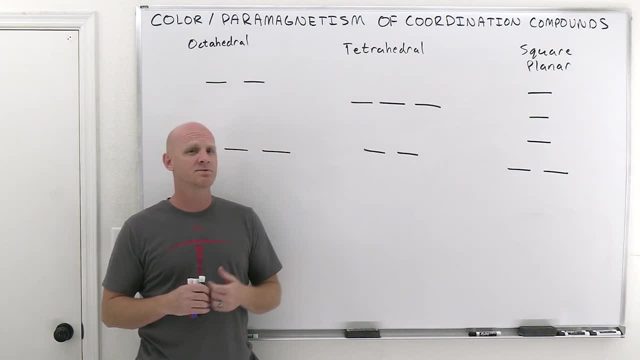 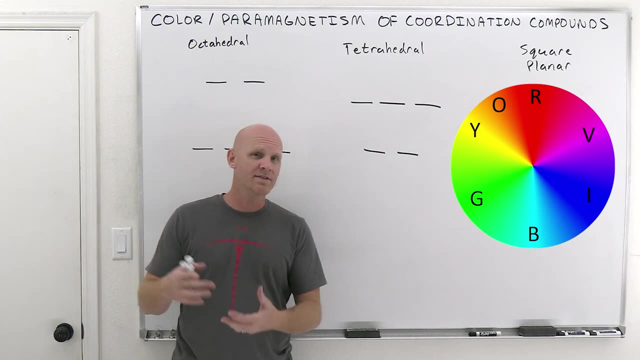 that's not the color. it's actually going to appear to you and I. There's something called the color wheel And if you absorb, say, red light, well, red light is on one side of the color wheel, And if you're absorbing that red light, then you're going to reflect back most of everything else. 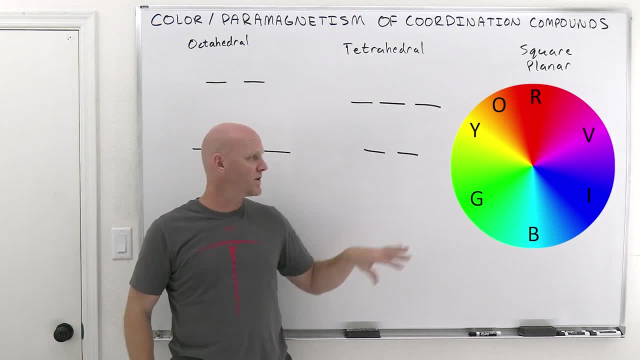 And the average of everything else would be on the opposite side of what we call the color wheel- And I'll put it up on the board here- And opposite of red typically, something going to be more in the green spectrum. So if it absorbs red light it's probably going to appear green in color to you and I. 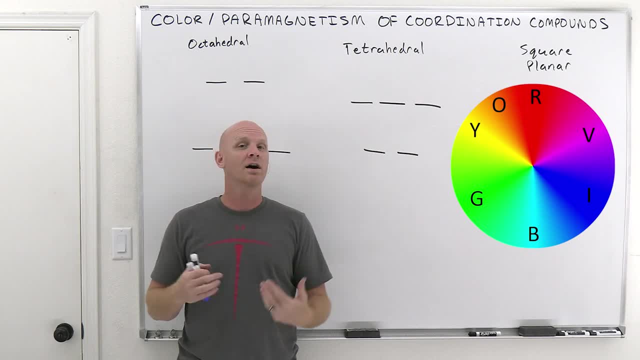 And so I just want to make sure you realize that the color it appears to your eyes and the color of light that's actually being absorbed are not the same color. We call them complementary colors, and they're on opposite sides of that color wheel. 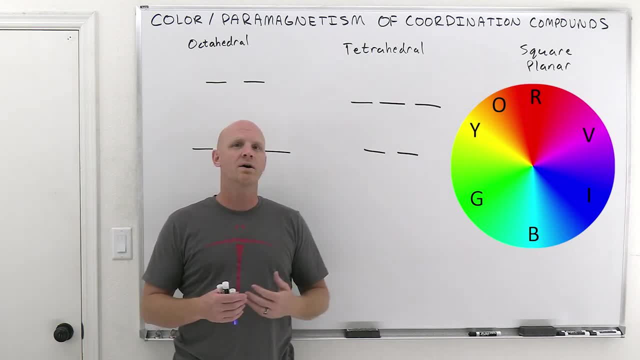 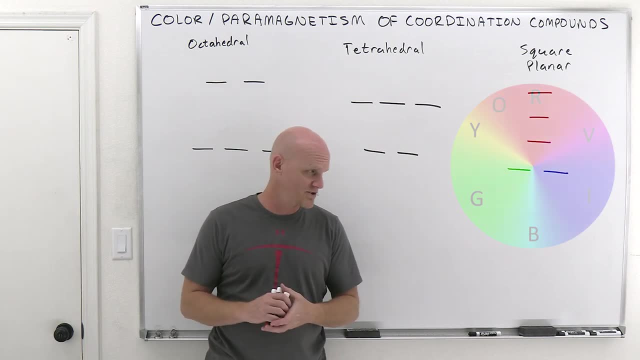 And so we will probably exclusively talk about the color of light being absorbed, not the color of light at which it appears to your eye, And I just want to make sure you realize that distinction here. All right, So it turns out a larger gap in energy. 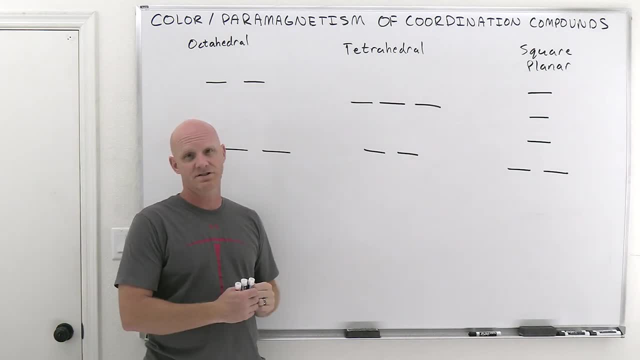 And these D orbital splittings is probably going to be shifted towards the violet end of the spectrum- the highest energy visible light and the smaller gap to be shifted towards the red end. red end of the spectrum And I say violet, but most of the time we just actually kind of call one end of the spectrum red and the other one blue. 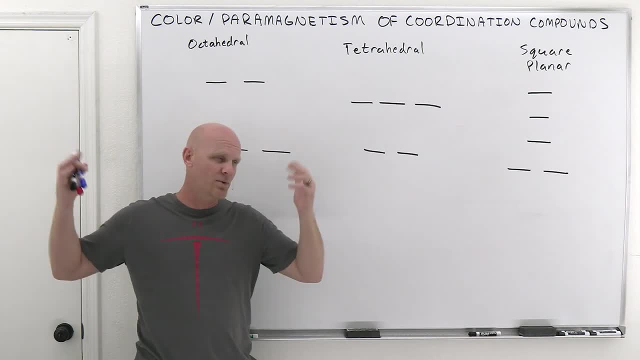 which notice it goes: blue, indigo, violet. So we really should call it the violet end of the spectrum. But for whatever reason, we often refer to red shifted and blue shifted, you know, depending on which end of the spectrum it shifted towards, and things of this sort. 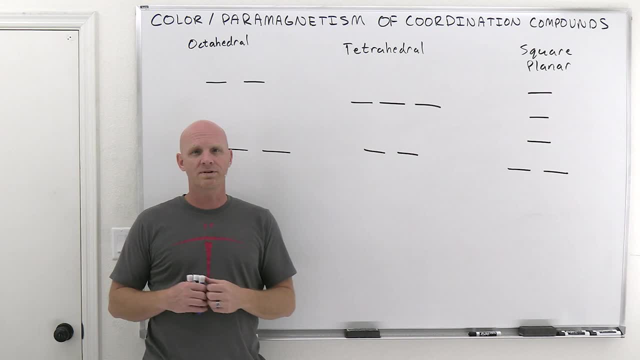 So just keep that in mind. So, but larger gaps absorbing light more towards the blue violet region. So, And then smaller gaps in energy between the D orbital splittings, going to be absorbing light closer to the red end of the spectrum. All right, 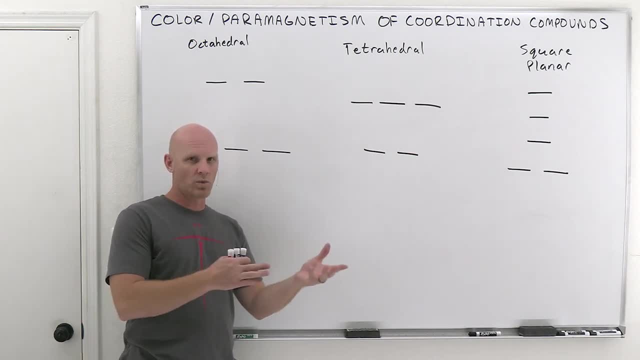 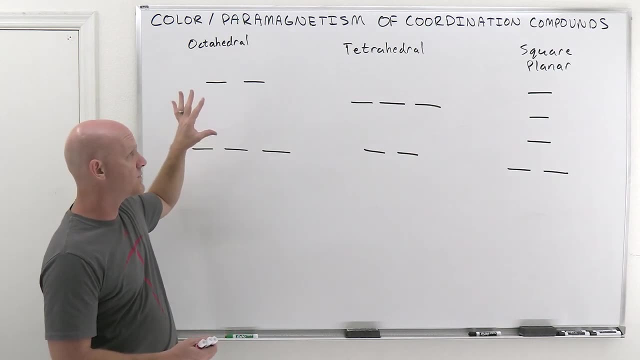 So we may not know the exact color, but at least we might be able to comparatively say it's more one way versus another, more towards the red or more towards the blue violet, if you will. Okay, So way this works then. requirement for being colored then: 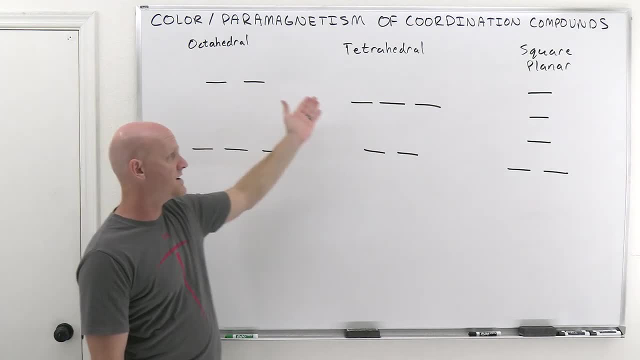 So is you got to be one of these D orbital complexes? And it doesn't matter if you're octahedral, tetrahedral or square planar, But the key is you have to have an electron down in one of the lower sets. 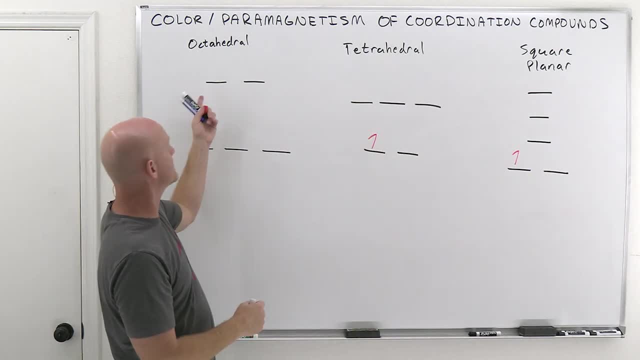 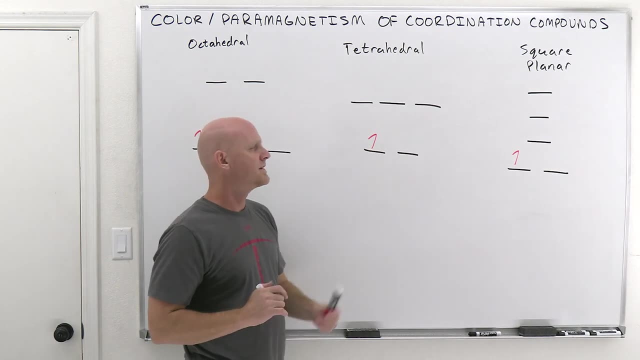 And then you have to have an empty place for it to go. One of these four spots in the octahedral or one of these six spots in the tetrahedral. And the square planar is a little bit special, If you recall, for a square planar they only exist for D eight. 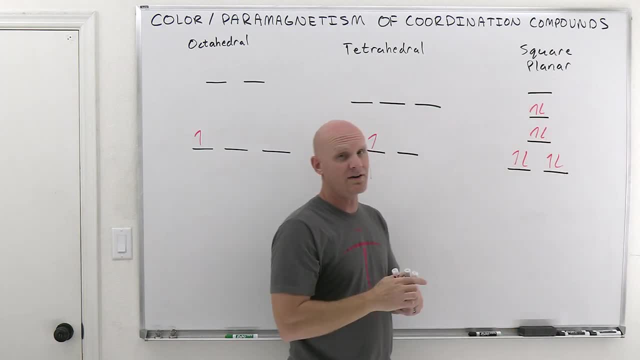 So these are always going to have eight electrons And so, square planar, we expect them to be colored all the time, because they're always going to have at least one electron- In this case, eight electrons, down here in one of these lower sets. 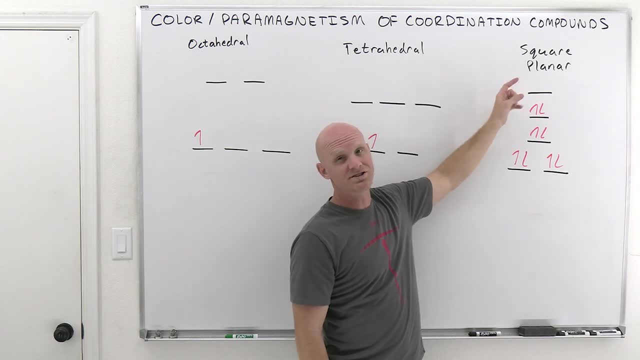 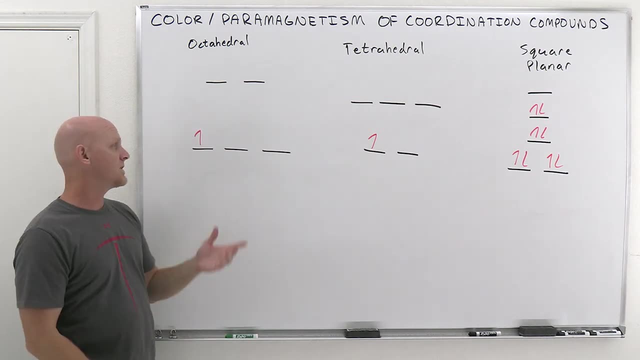 And they're always going to have an empty spot. In this case it's got two empty spots in that highest energy orbital, in the D orbital splitting, And so for a square planar, Yes, we expect them to be colored. Now for octahedral. so here with one electron in the d orbital. 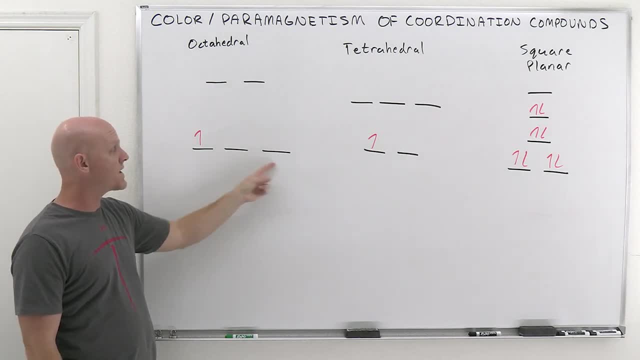 yeah, I've got an electron in one of these low energy orbitals and I've got four empty spots up here to which it could go to, and so if it absorbs light of just this energy difference, this same energy as the crystal field, splitting energy, 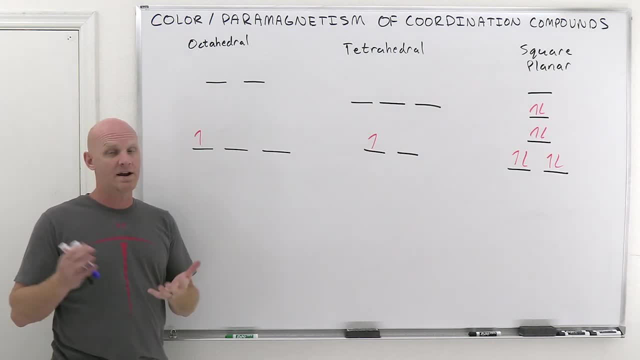 well then, it's going to absorb visible light in all likelihood, and appear colored to the naked eye. So when would we expect maybe an octahedral or tetrahedral complex not to be colored? Well, I'll give you an example. So if you have a metal ion that is d0, no d electrons, 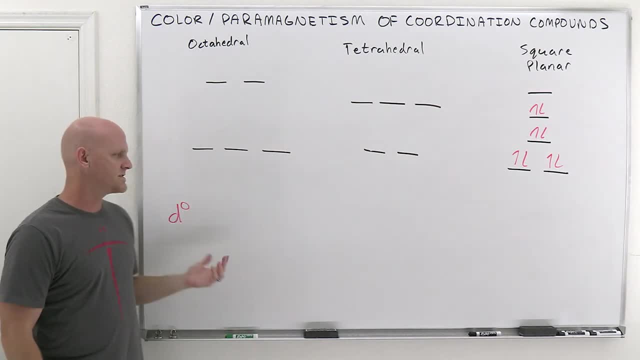 well then there's no electrons down here or here and, as a result, you don't have any electrons that could get promoted up to the higher set of d orbitals. So if you're d0, no guarantee you're going to be colored. 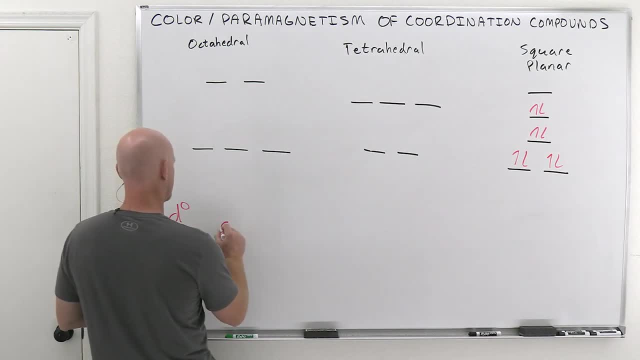 We don't necessarily expect you to be colored, So other side of the coin is going to be d10.. And so d10,, whether you fill it in, low space, spin or high spin, and in this case I'll do it with the octahedral here. 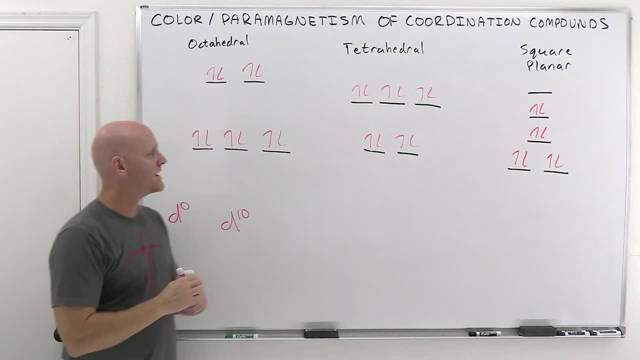 and then the tetrahedral here and notice. in either case, I do have electrons now down in these lower energy sets of orbitals, but I don't have a place for it to get promoted in the upper set because they're full as well. 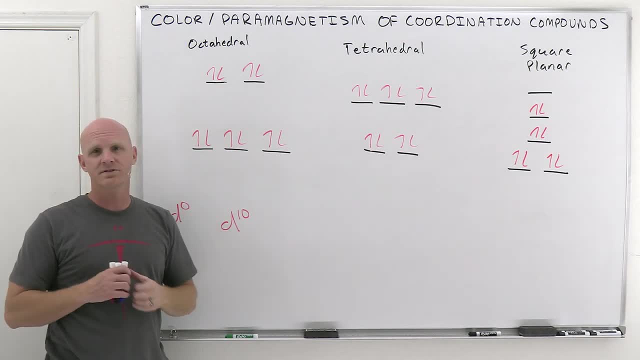 And so for d10, no reason it should be absorbing light corresponding to the crystal field splitting energy. no reason we'd expect it to be colored Now it could be colored for other reasons, It turns out this d orbital splitting is not the only reason. 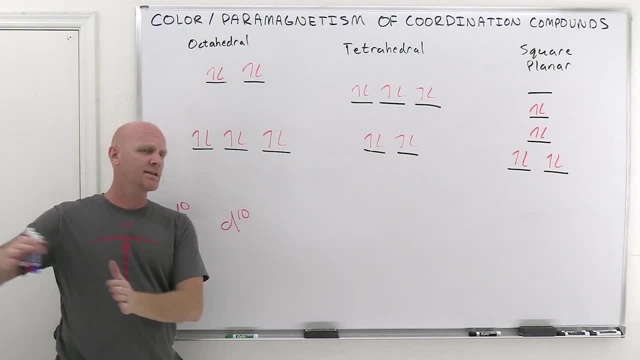 so that compound's going to be colored, and if you take organic chemistry, you'll learn about pi, electrons and things of this sort. So, however, in this chapter, this is the principal reason why things might appear to be colored. And so if you have d1,, 2,, 3,, 4,, 5,, 6,, 7,, 8, or 9,, 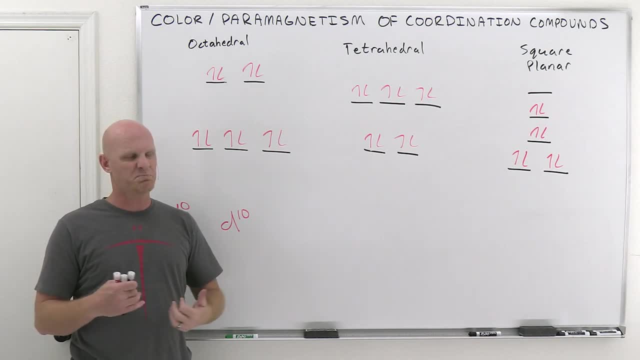 we should expect that compound to be colored. Is it guaranteed? No, Is it pretty likely? Yes, But if you're d0 or d10, we probably are going to expect it to be colorless and not be colored. Is that guaranteed? Well, no, 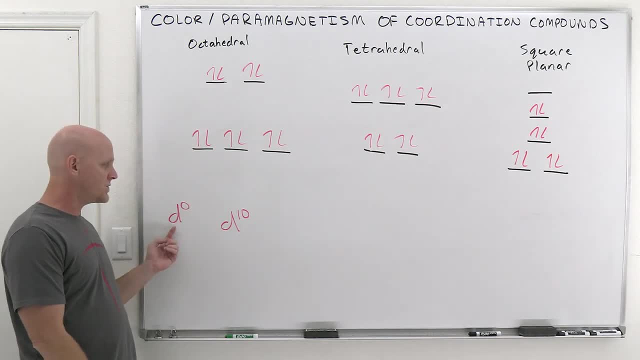 But again, it's just part of the trend: Really high likelihood that something with no d electrons or 10 d electrons is going to end up being colorless. All right, So that's color. Now we've got to talk about what we refer to as paramagnetism and diamagnetism. 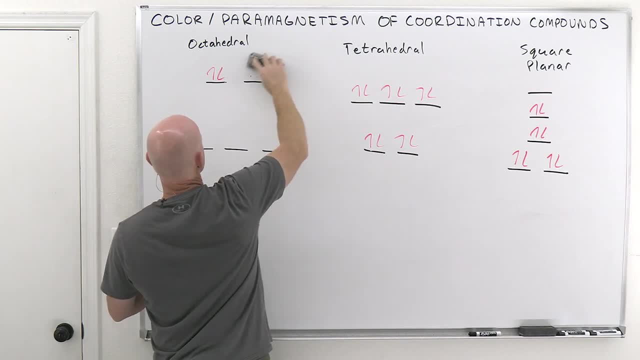 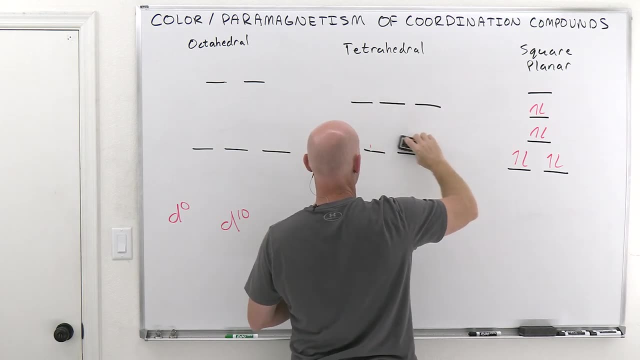 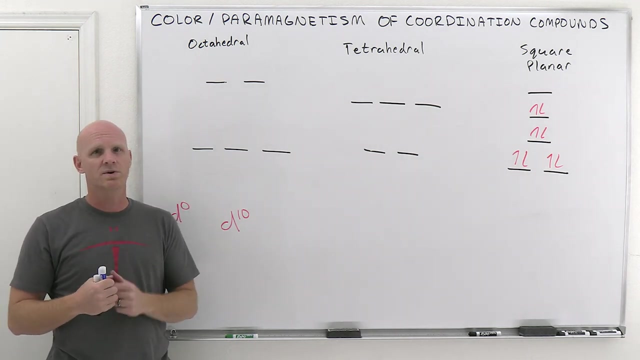 Empty these out a little bit And so these are going to be different than ferromagnetism kind of the magnetism we associate with iron And that deals with you know little areas of iron where you've got spins kind of aligned and things of this sort. 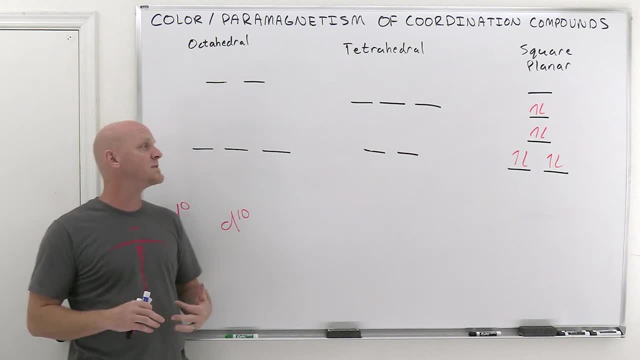 And we're not going to go there, But this is related. This is related to spin, but it's going to be the spins typically of unpaired electrons. It turns out, electrons have a spin associated with them And we like to say either spin up or spin down. 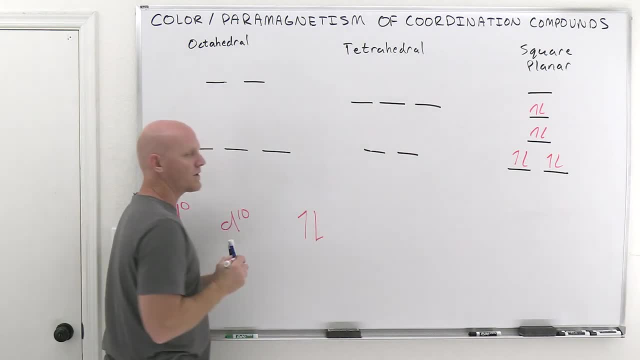 And that's when we write electrons. you know we like to represent that with an up arrow or a down arrow, But there are two opposite spins And they are exactly opposite in magnitude as well. And so it turns out when you pair up electrons. 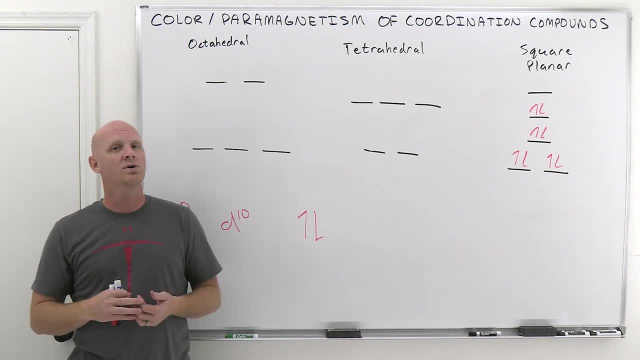 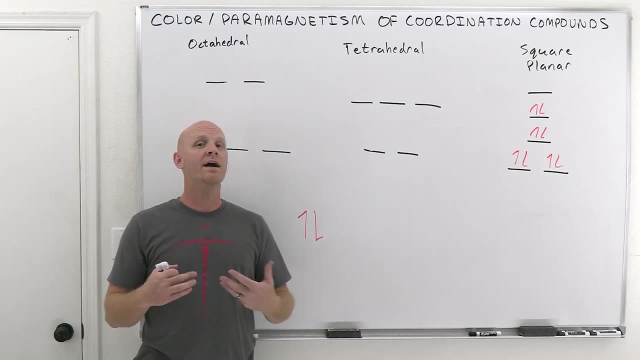 their spins cancel each other out, And so to have an overall spin associated with an atom. here you've got to have unpaired electrons, And it turns out that leads to a state we call paramagnetism. We say that that substance is paramagnetic. 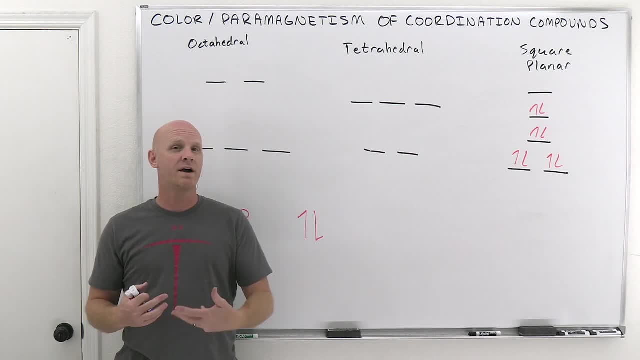 And that's the requirement. You've just got to have unpaired electrons. And it turns out, the more unpaired electrons you have, the more paramagnetic it becomes. Well, what does this ultimately mean in terms of magnetism? Well, it means that if you have one of these lovely complexes, 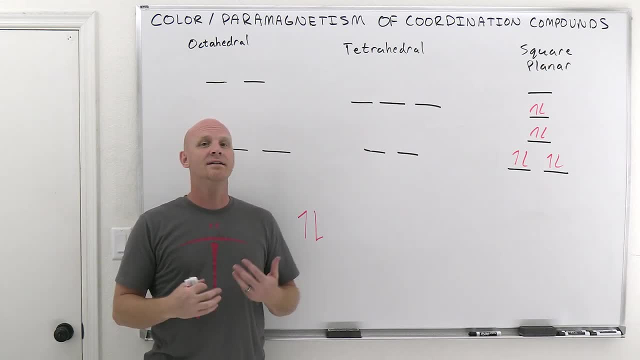 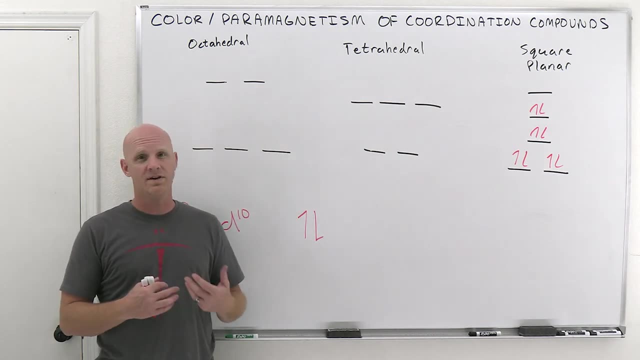 or metal ions or whatever, moving through a magnetic field. it's going to experience a slight attraction as a result, And the more paramagnetic it is, the more of that attraction it's going to feel. Now, on the other hand, what if all the electrons are all paired up? 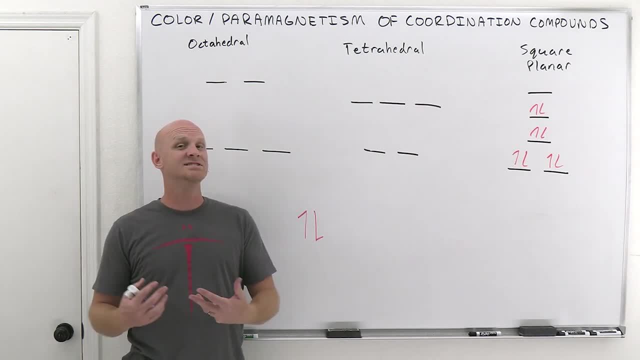 Well, if the electrons are all paired up, we would refer to it as being diamagnetic instead, And in this case, instead of experiencing a slight attraction, it's going to experience a very, very, very, very, very slight repulsion instead. 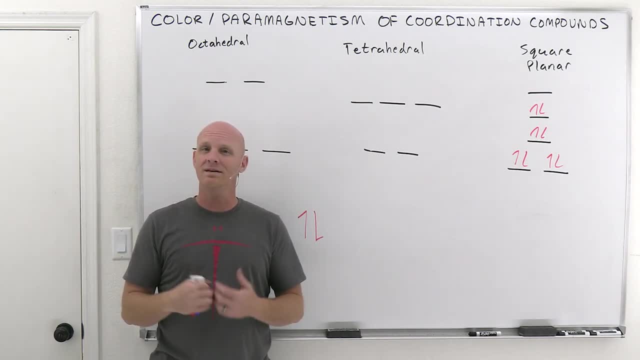 But because all the electrons are paired up, there's no net spin, And that's why it's going to end up not having this paramagnetism associated with it. And so you're going to have to look at this. You're going to have to look at the number of d-electrons. 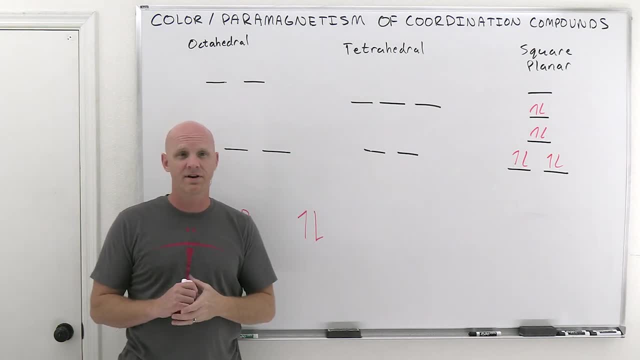 and you're going to have to fill them into one of these diagrams, depending on what kind of complex you're told you have, and just figure out: do I have unpaired electrons, yes or no? If yes, well then that's going to be a paramagnetic complex. 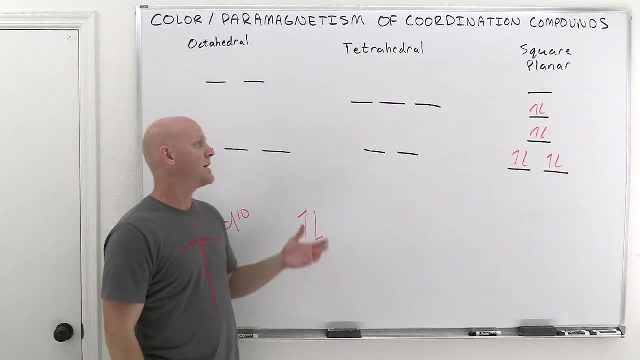 And if no, well then that's going to be a diamagnetic complex. And so by simply looking at the number of d-electrons now and how they might fill in on the type of complex you have, we now have a way of evaluating whether it's colored. 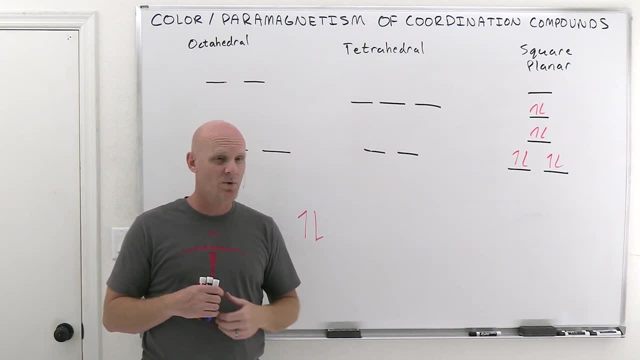 or whether it's going to be paramagnetic or diamagnetic, And those are the kind of questions we're going to answer here. So let's take a look, All right. so the first one we're going to take a look at here is SC3+. 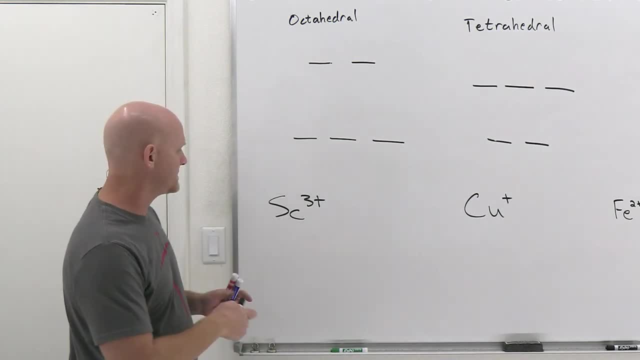 And first order of business is you just have to figure out how many d-electrons we're dealing with, And so scandium is going to look like argon 4s to 3d1.. So if you recall, in the crystal field theory lesson we went right back over. 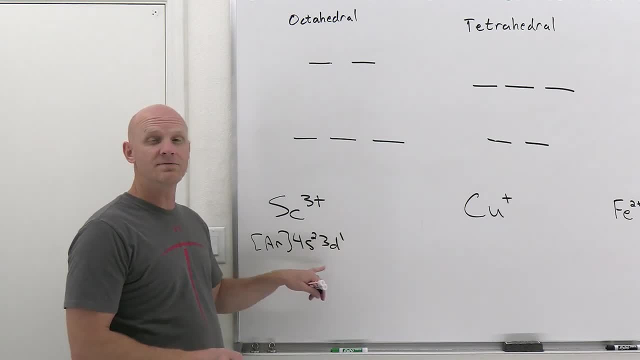 We started off by figuring out electron configurations, reviewing it a little bit so we could figure out these number of d-electrons, And this is definitely one of the examples we went over. So this is scandium, but scandium 3+, we're going to lose three electrons. 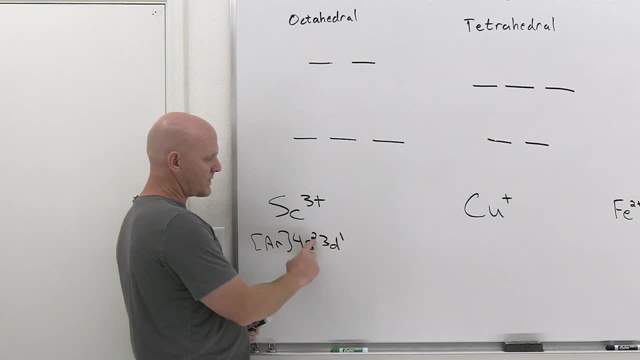 Well, you lose the s's, before the s's, You lose the d's, but that's two that we have to lose for the s's and then one d, And all we're going to have left with is just plain old argon. 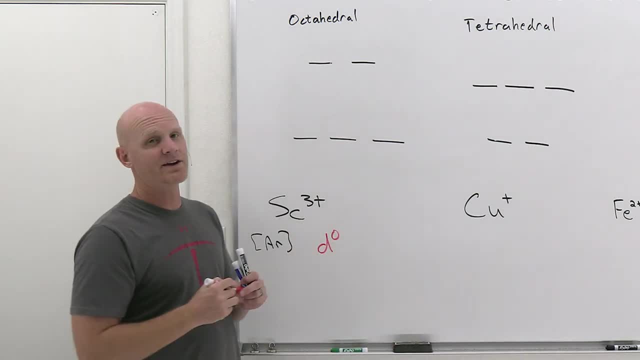 And what this ultimately means is that scandium does not have any d-electrons at all, And so, in this case, if you had to choose, would you expect it more likely to be colored or colorless? Well, with no d-electrons, no electrons that can be promoted. 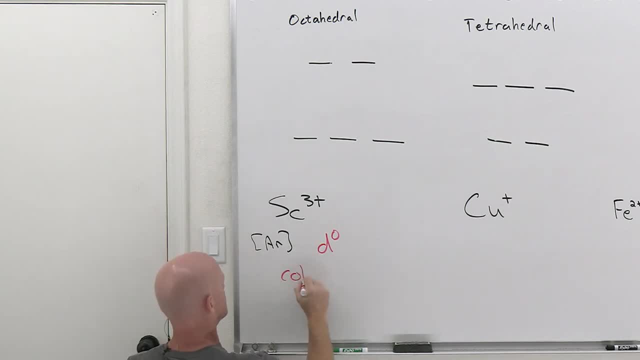 from the lower set to the upper set. we'd expect it to be colorless And then paramagnetic or diamagnetic In this case if you're isoelectronic, to argon or noble gas where you've got a filled octet in that last shell, and stuff like that. 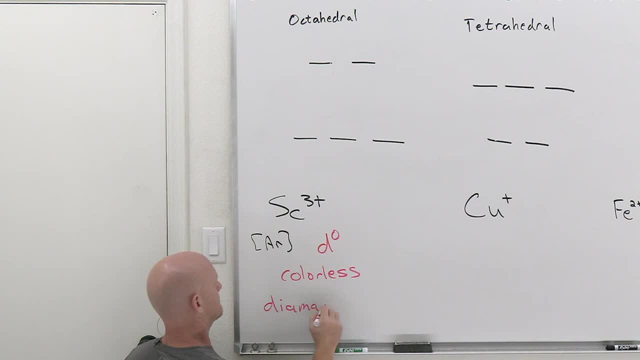 all the electrons are going to be paired, And so you're going to be- I can spell this- diamagnetic. All right, so that's SC3+, Moving on to copper plus, And recall that copper is one of those lovely exceptions. 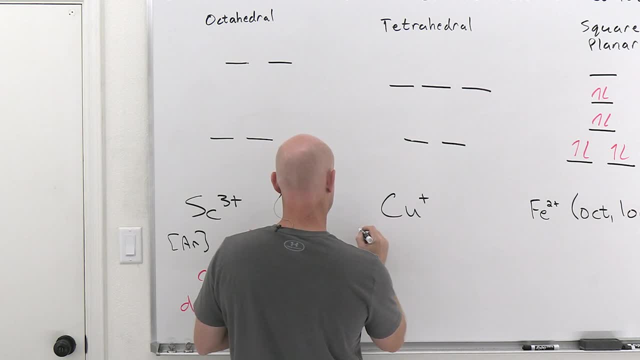 And we've got the electron configuration now for copper, argon, And instead of 4s2, 3d9, you've got to remember that copper is argon 4s1- 3d10.. But again we don't have copper. 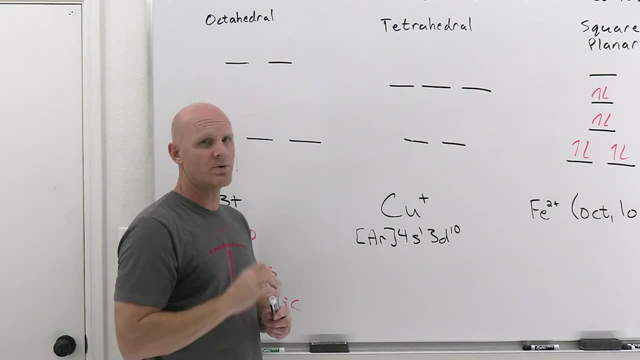 We have copper with a plus one charge. We've got to remove one electron, And in this case you've got to remember that you remove electrons from the 4s before the 3d, And so we're going to lose that one electron right there. 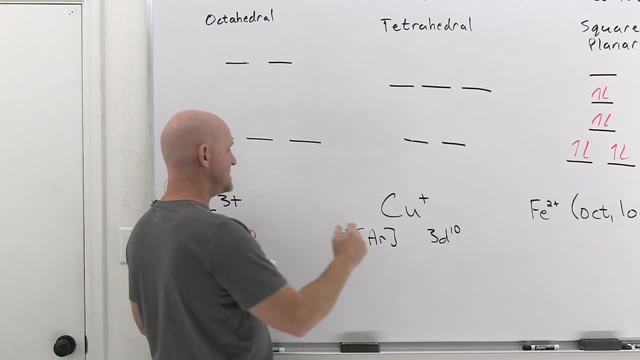 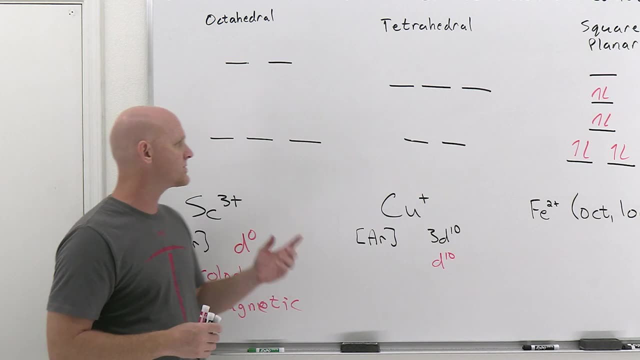 and we're just going to have argon 3d10.. But the big deal here is that we have 10 d-electrons. That's what we really need to figure out. Well, with 10 d-electrons, these are all full. 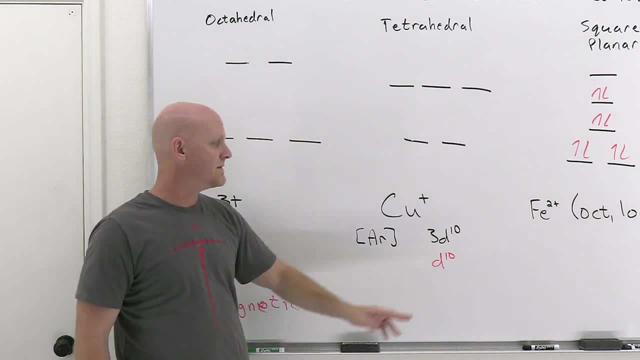 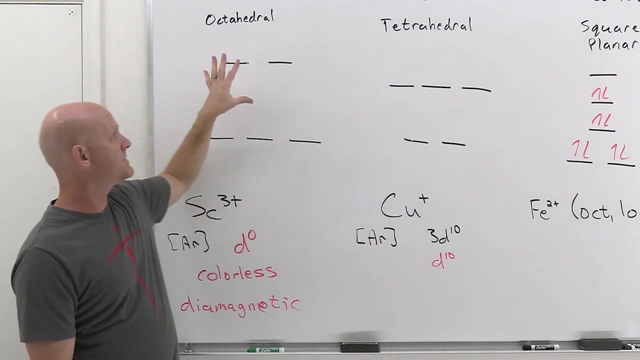 So notice, I didn't tell you if it was all full. If it was octahedral or tetrahedral With 10 d-electrons, you'd know it's not square planar, because those only exist for d8 complexes. But with 10 d-electrons it didn't matter if you fill in. 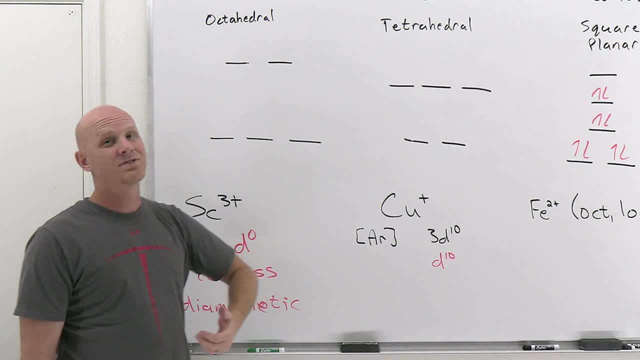 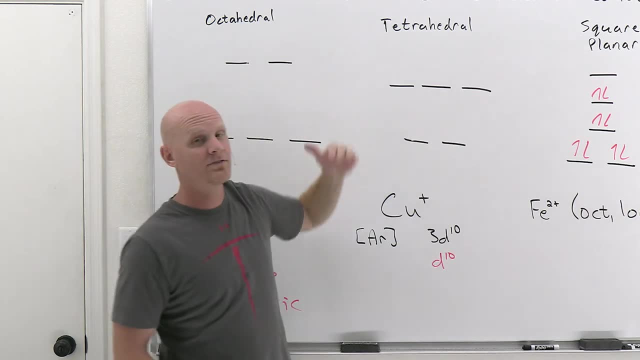 the octahedral or the tetrahedral, They're going to be full either way. And if they're full either way, well then there's no empty spots up here for the electrons down here to get promoted to. And so if I had to pick- if it's more likely to be colored or colorless- 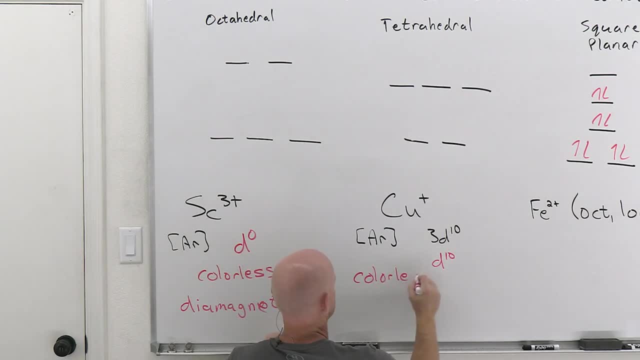 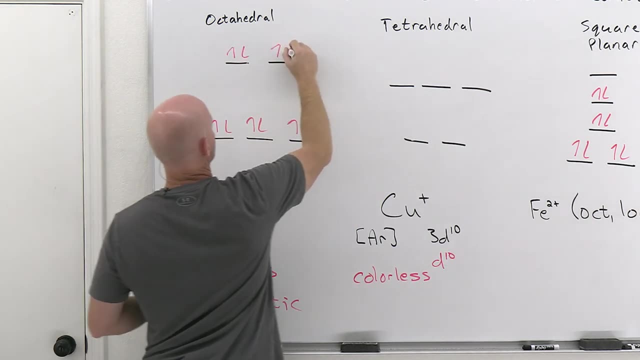 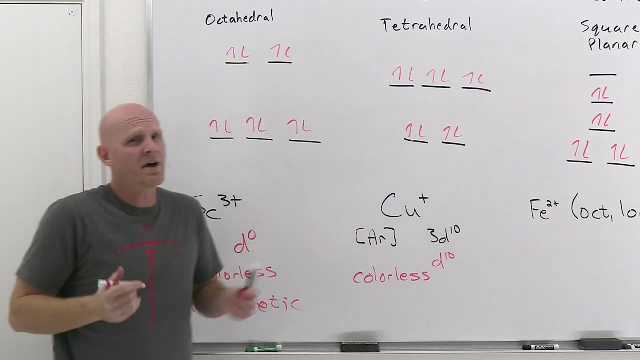 I'm going to pick colorless. And also, if we fill these in again, you'll see that, regardless of whether it's octahedral or tetrahedral, they're all paired up, all of them. And if there's no unpaired electrons, 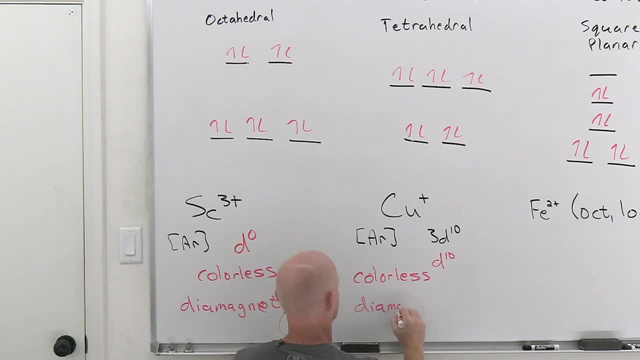 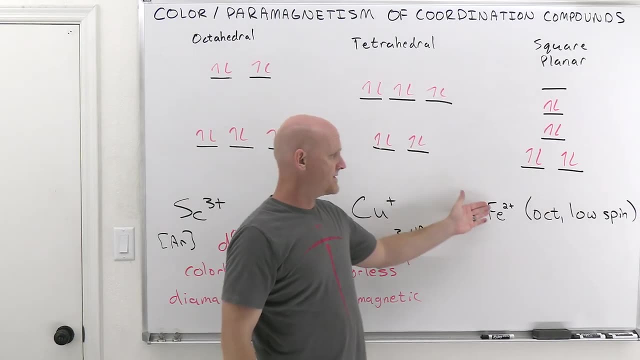 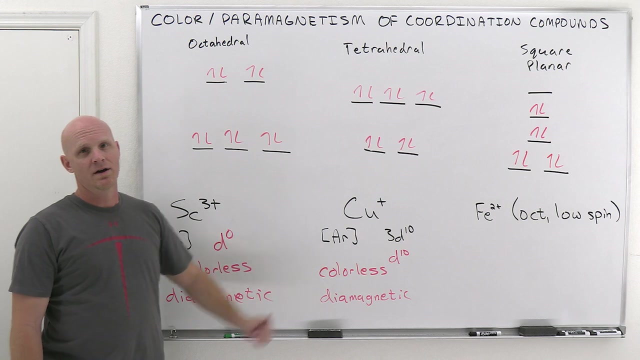 then we're going to expect it to be diamagnetic. All right, moving on to Fe2 plus here. And so Fe2 plus, and notice here I specified it's octahedral low spin. And notice I didn't specify that on the last ones here. 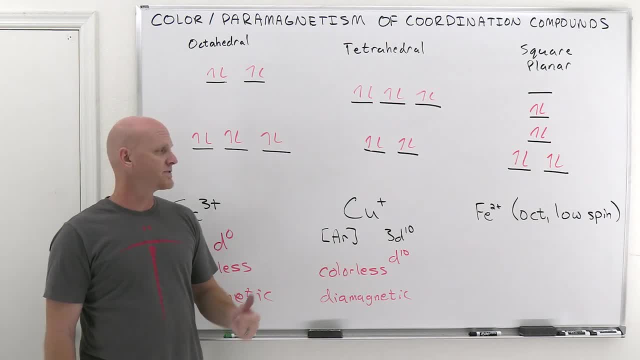 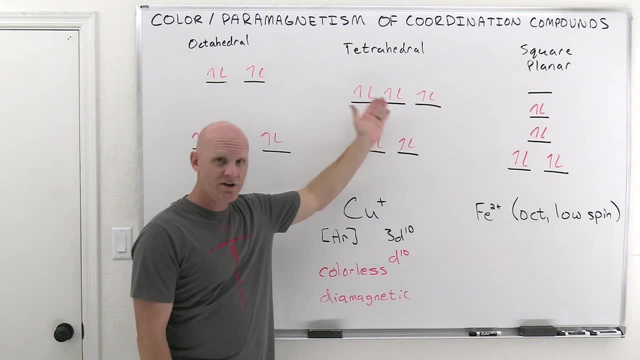 because with either zero electrons or 10 electrons it wouldn't make a difference. But Fe2 plus, it turns out, is going to end up being d6, and it's going to totally make a difference how you fill them in, whether it's tetrahedral or whether it's octahedral low spin. 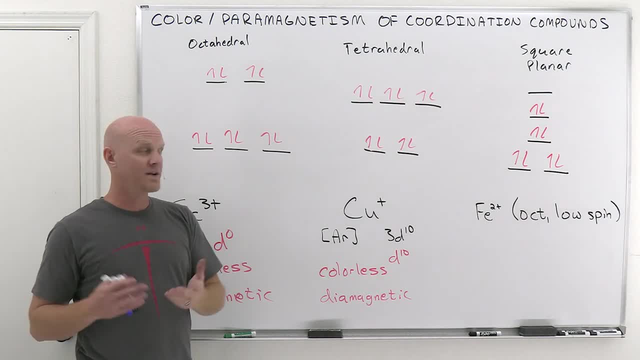 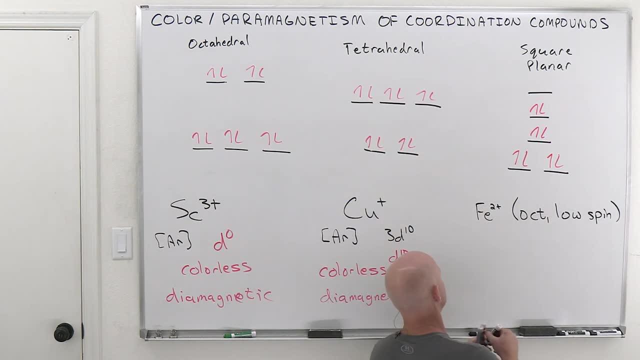 or octahedral and high spin. But with 60 electrons we'll find out again. it can't be square planar, But three options, so I had to tell you which of those three it was going to be. So let's figure this out though. 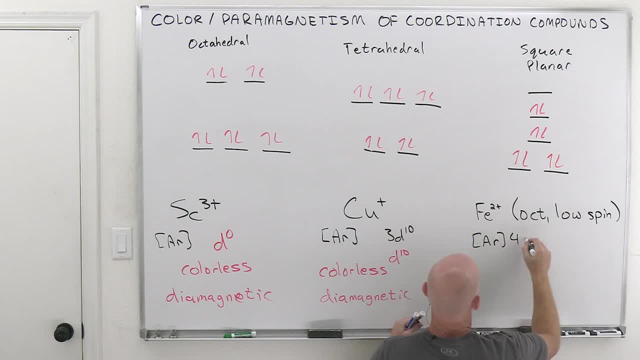 We've got again. iron is argon 4s2, 3d6, but we need to lose two electrons And so, again, you remove the s's before the d's, So it's just going to be argon 3d6.. 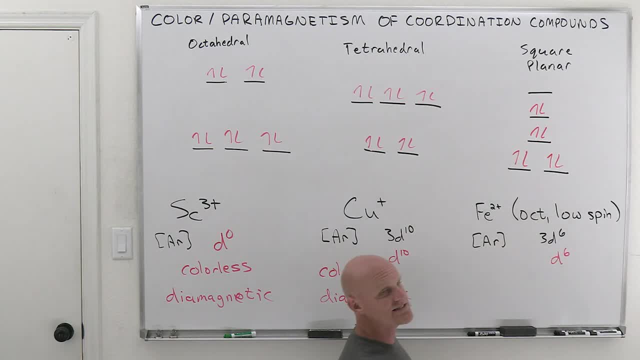 And so, once again, the key here is that we've got 6d electrons. That's the important part. And now we've got to look and say, okay, because there's 6d electrons, it's low spin, octahedral, Let's fill those in. 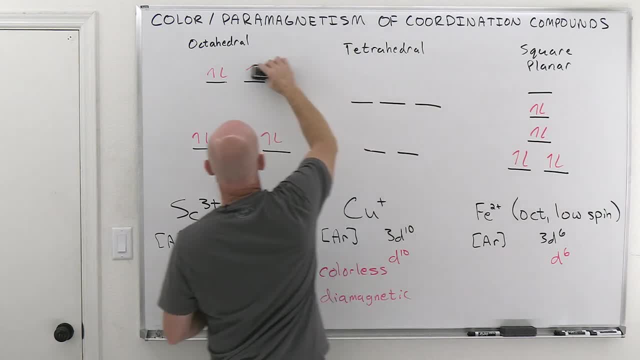 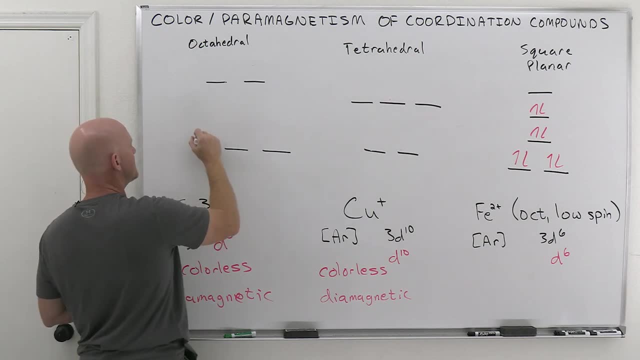 Let's take a look at what that looks like here. Let's empty these back up, Okay, so in this case 6 electrons. low spin means we fill up everything down low before we ever go up high. So this means we have a very large crystal field splitting energy. 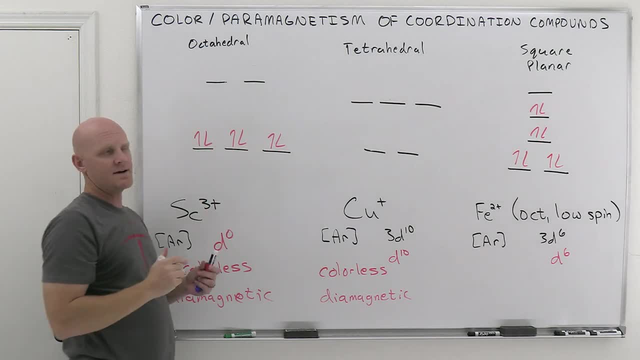 and so it's easier to pair the electrons up down low than to bump them up up high. So in this case, we filled in those 6d electrons and we can see that, yeah, we totally expect this thing to be colored. 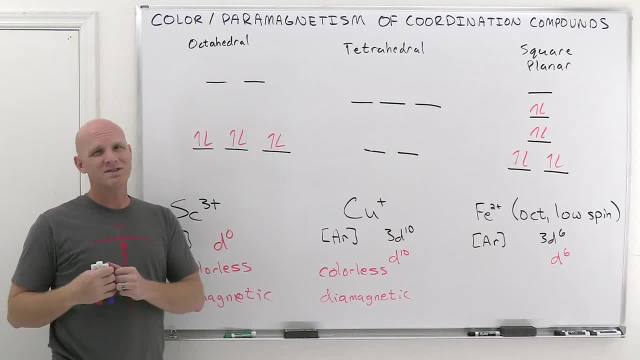 But again, typically d1 to d9, you expect those things to be colored. Now some of you might learn an exception for things that have 5d electrons, and they're all unpaired. If you want to promote it, we have to switch its spin, which is a rare event. 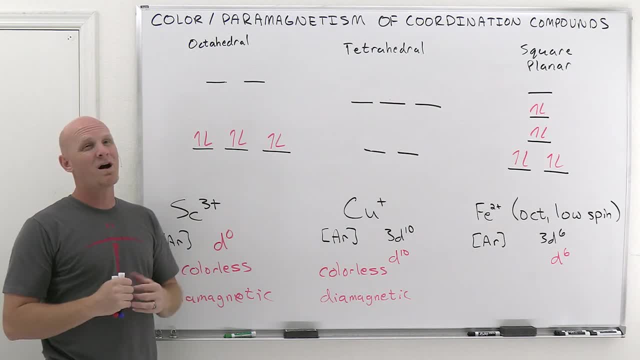 And if you learn that, well great, then you're probably on the hook for that, But most of the rest of you, you're probably just going to learn about the two extremes, where if you're d0 or d10, probably colorless, d1 through d9, colored. 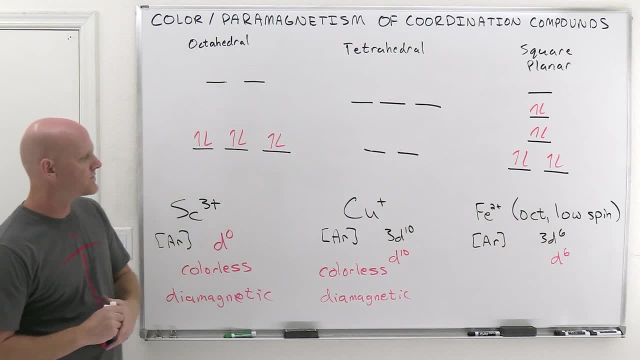 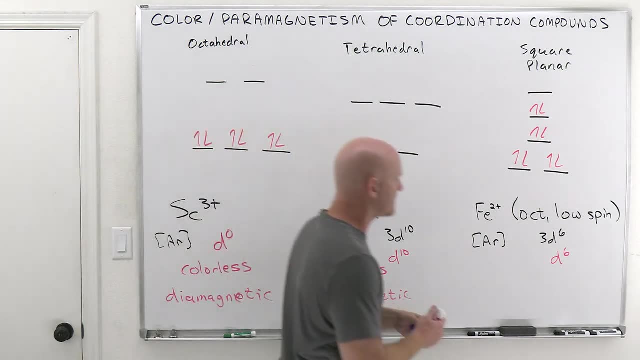 If you've learned that d5 exception, I'll leave that to you, but not something most students are normally presented with at this level. Okay, so in this case, because it's d6, if I had to pick colored or colorless, 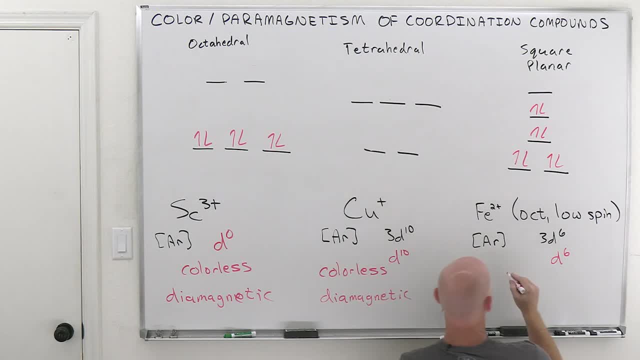 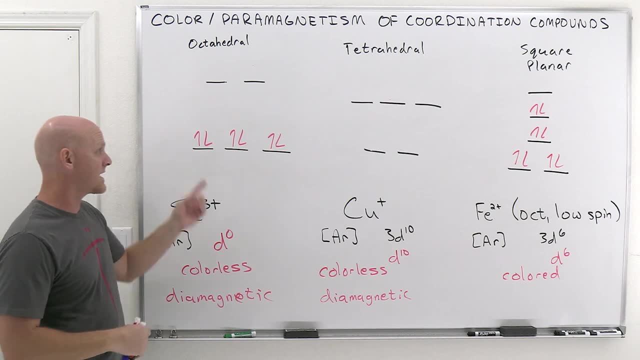 I'm definitely picking colored. I've got electrons down there that could get promoted up to a fraction of visible light, So we'd expect to be colored. And then, as far as paramagnetic, diamagnetic, I can see that all the electrons are paired, all of them. 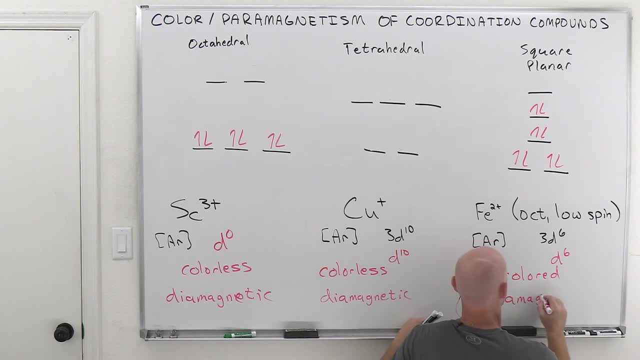 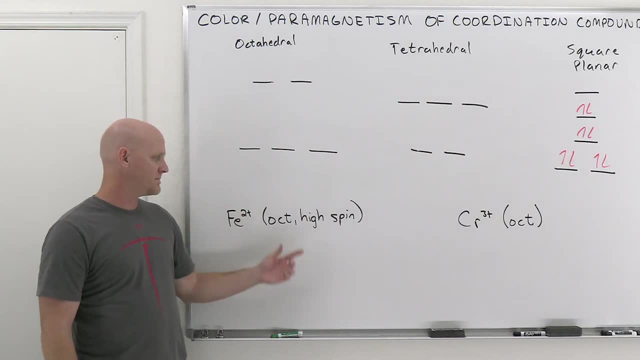 And so it's going to end up being diamagnetic. All right, so our next example here is Fe2+, But instead of being octahedral and low spin like the last example, it's now going to be octahedral and high spin. 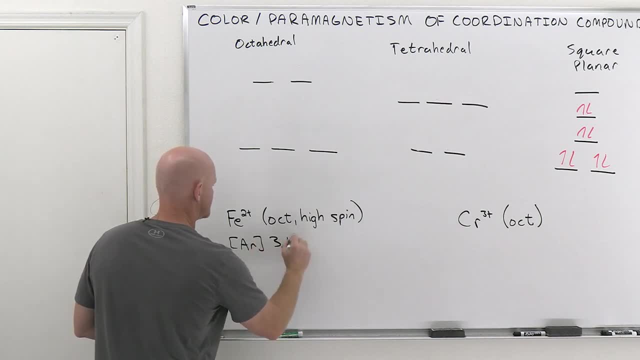 Well, we already figured out that Fe2 plus and electron 3d6, we lost the two 4s electrons to become 2 plus. So same as the last example we did So big thing again here is that it's 6d electrons. 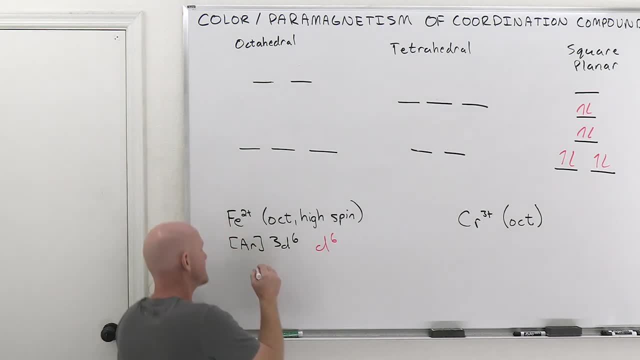 And having 6d electrons, so we'd expect it to be colored rather than colorless. So, and if we fill in those in a high spin fashion, here we'll see why. So, filling in 6d electrons, so 1,, 2, 3.. 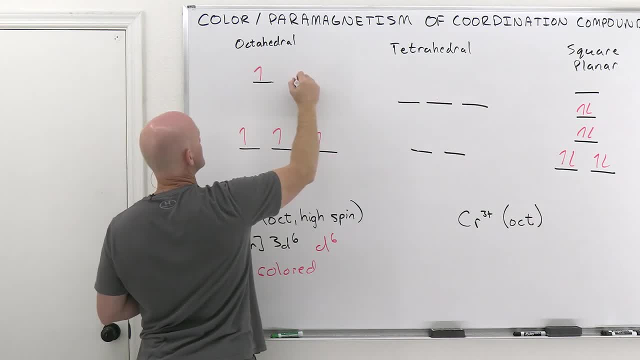 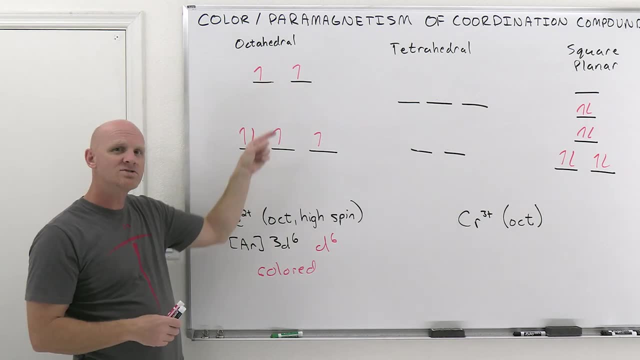 And if we fill them in high spin, you go up high before pairing up anything down low. So 4,, 5, and then 6.. And so now we've got 4 electrons down here, And I still have two empty spots up here to which they could go. 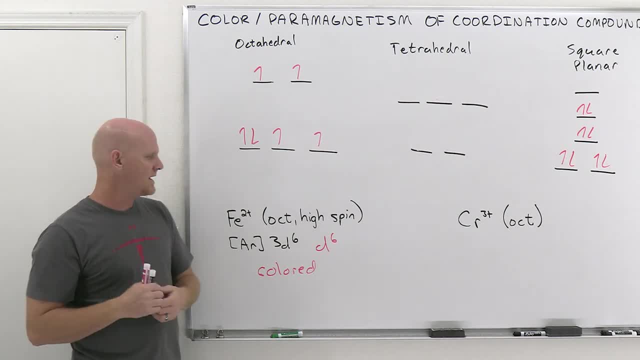 And so, yes, we'd expect it to be colored. And again, usually d1 to d9 we expect to be colored. Now, as far as paramagnetic or diamagnetic, we can see that we've got 1,, 2,, 3, 4 unpaired electrons. 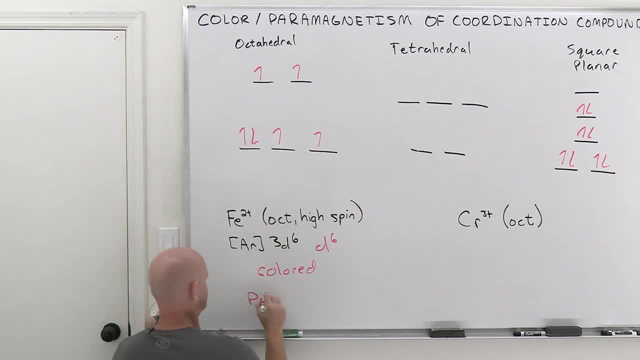 This thing is very paramagnetic as a result. So Fe2 plus makes a really good comparison in this regard because, as we saw, with the Fe2 plus low spin all the electrons were paired and it was diamagnetic, But with the Fe2 plus high spin, 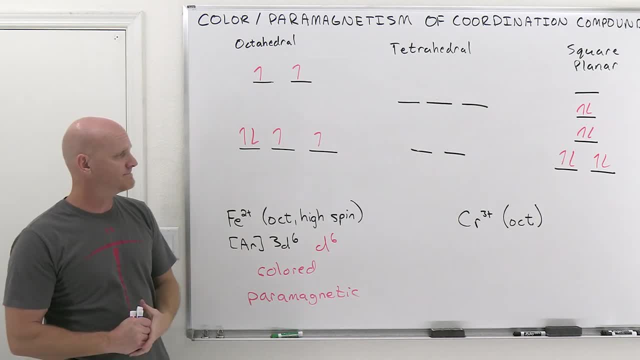 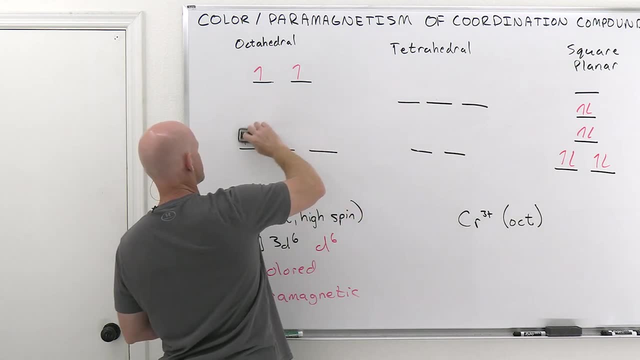 so we had 4 unpaired electrons and it ended up being paramagnetic instead. All right, Cr3 plus. And so if we take a look at Cr3 plus now and erase our electrons here from the last example before we get started? So, but again, you got to remember that chromium is one of your exceptions here. 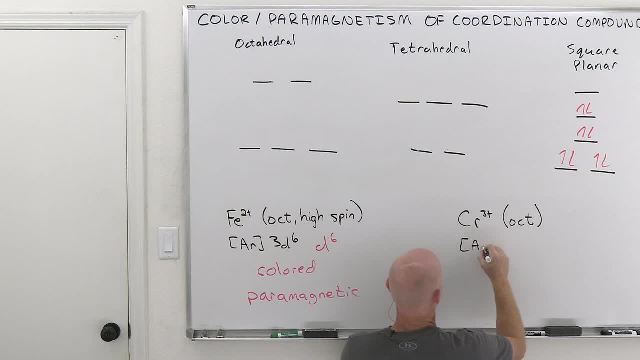 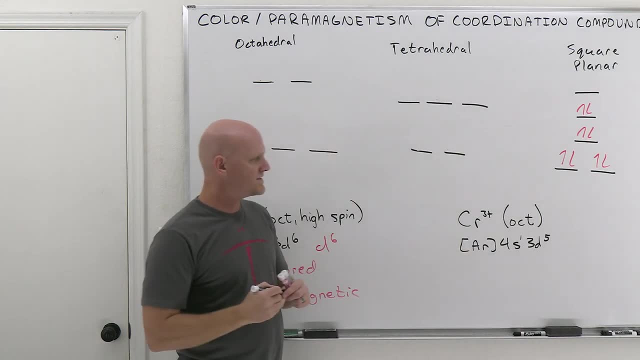 And so chromium is electron. configuration is argon: 4s 1, 3.. 4s 1, 3, d5. So instead of s2d4, it's s1d5. Promotes one from the 4s to the 3d to get them both half filled here. 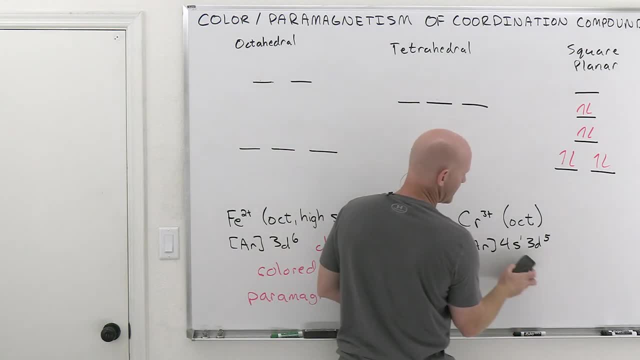 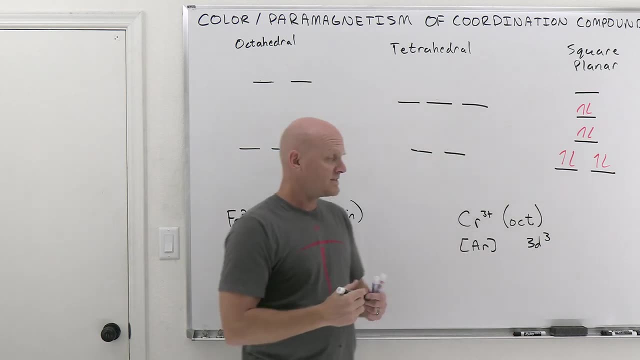 And now we got to lose three electrons. Well, we're going to lose that 4s electron first, And then we got to take away two more to become 3d3.. And notice this: didn't say if it was low spin or high spin. 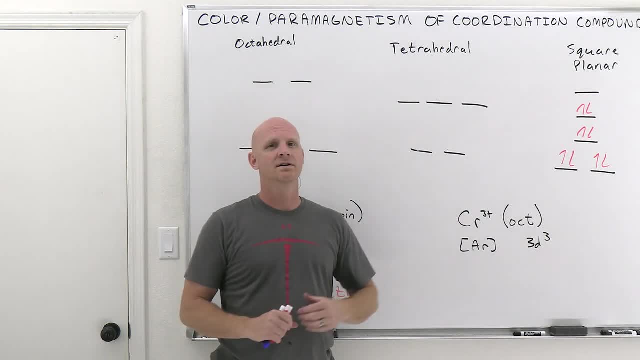 It's because it didn't have to. You got to have between 4 and 7 inclusive d electrons to have distinct low and high spin Cases, So complexes, And so in this case, with d3, whether you filled it in the low spin way or high spin way. 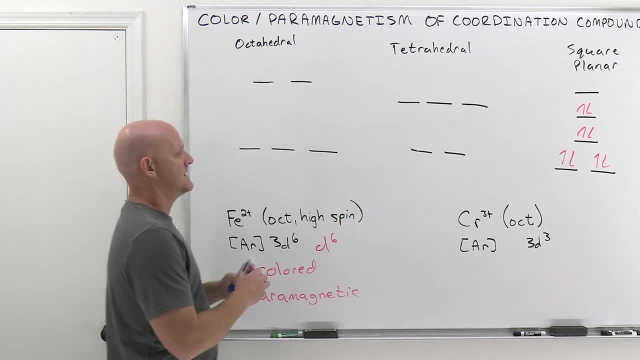 it's going to look exactly the same And so it doesn't make a difference. So I didn't have to specify, And so in this case we fill in 3d electrons 1,, 2, 3.. We see what that's going to look like. 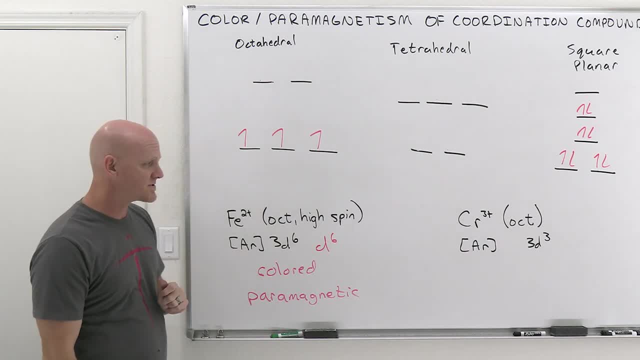 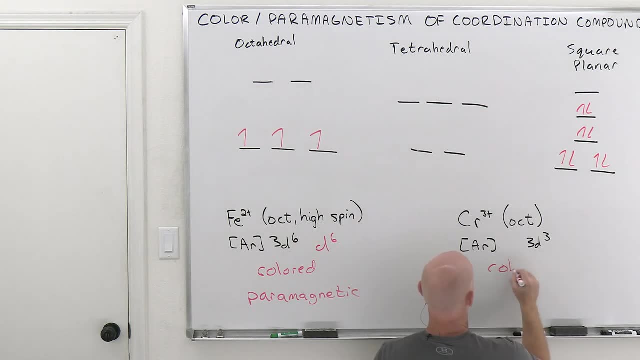 And whether this had been filled in the low spin way or the high spin way, it looks exactly the same for those first three electrons, Again, that's why it doesn't matter. But again, having d electrons but not being full, we expect it to be colored. 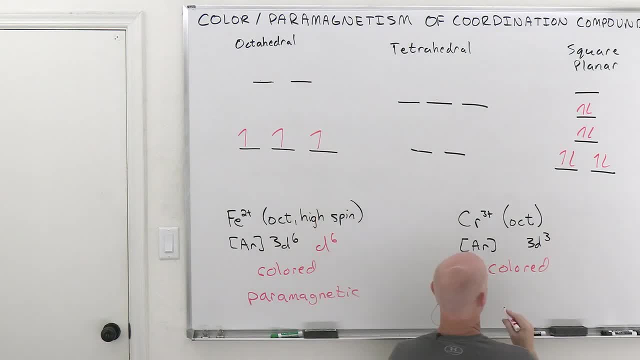 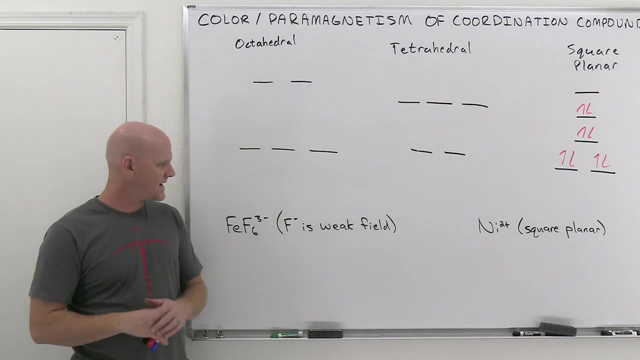 We definitely have electrons in that lower set that can be promoted up to the higher set- Empty spots- And then we see that we've got three unpaired electrons And so we'd expect it to be paramagnetic. All right, So last couple examples here on this question. 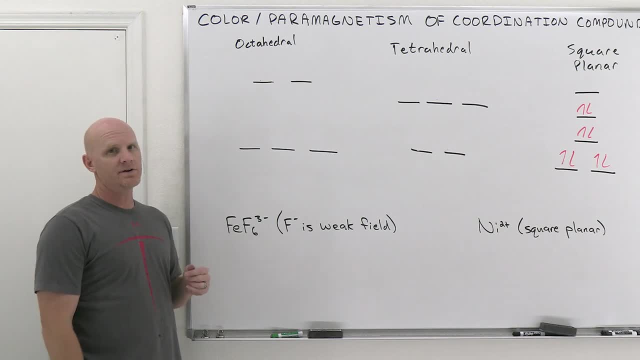 So in this case we're given an entire complex here And you got to figure out. well, okay, There's six fluorines there. They're monodentate ligands. This has got a coordination number of six, So it's got to be octahedral. 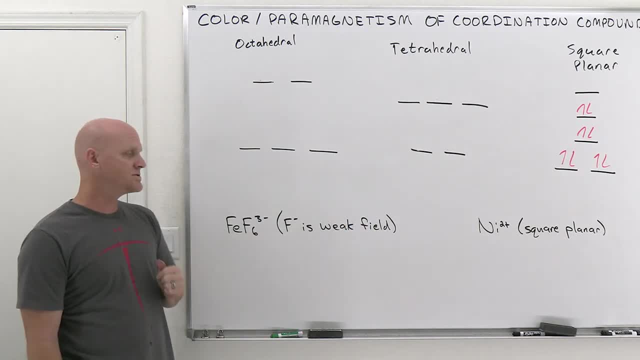 It didn't tell you that it was octahedral, But from the formula of the complex you can deduce that it's octahedral. But in this case, instead of saying is it high spin or low spin, I told you that F minus is weak field. 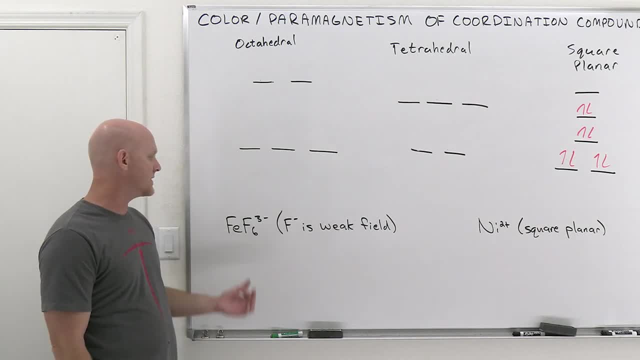 Okay, So this is a little more challenging question, A little more things to figure out here. Well, first off, we've got to figure out what's the oxidation state of Fe here. Well, in this case, the fluorine, the fluoro ligands, are minus one each. 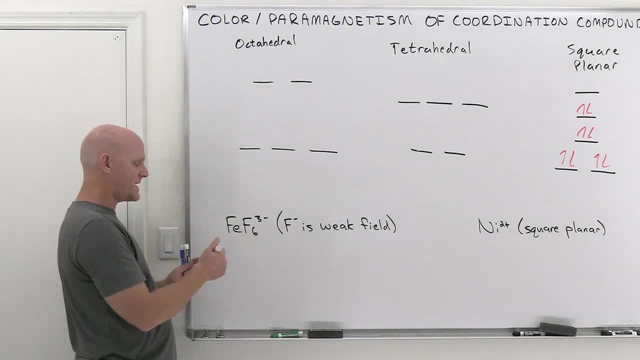 And there are six of them for a total of minus six. So if the whole complex is minus three, then the iron here has to be in the plus three oxidation state, And so if we take a look at Fe plus three, recall that iron again is argon 4s2.. 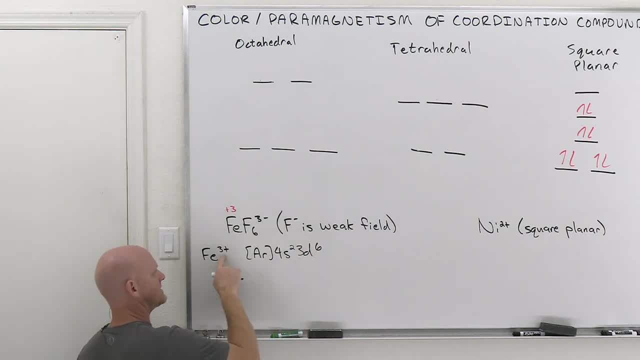 3d6. But if we're at Fe3 plus, we got to lose three electrons. The first two we lose are the 4s's, And then we'll lose one of the 3d's, And so, in this case, 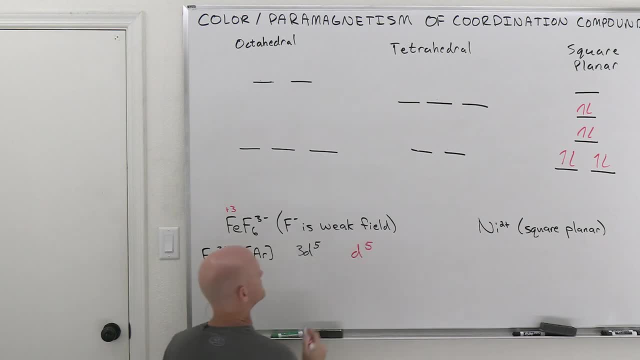 the big key is that this has 5d electrons. Okay, Now again, instead of being told it's low spin or high spin, you're told that it is weak field. So you got to recall that weak field corresponds to a small crystal field splitting energy. 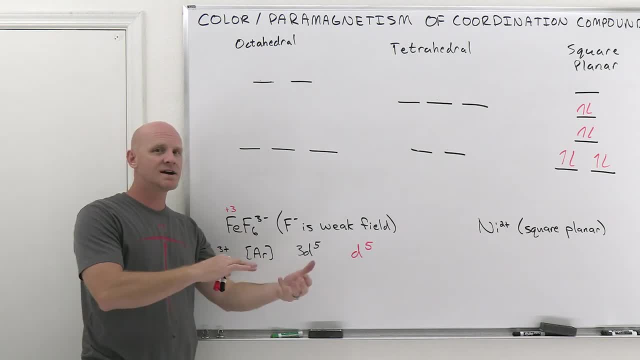 which corresponds to a high spin. So weak field goes with high spin, strong field goes with low spin. So when you see weak field you're supposed to think, oh, that's going to be high spin, And so high spin again. 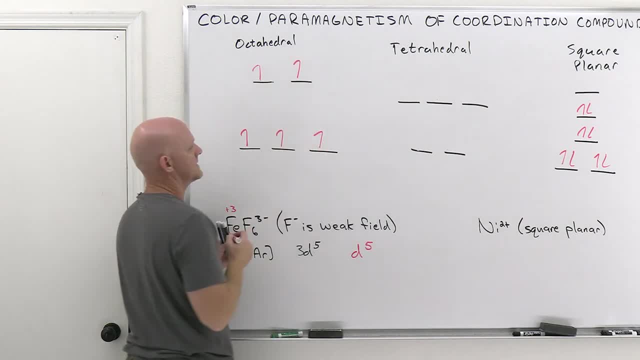 means we go up high before we pair anything up. And so there's your d5 and we got five unpaired electrons, And we can definitely see in this case that it's likely to be colored. for most of you, However, it's not a given here that it's going to be colored. 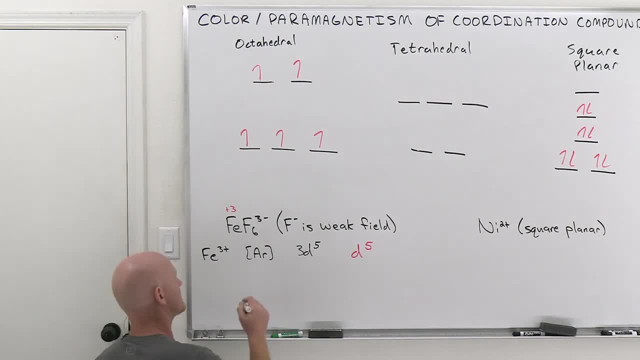 it turns out- But I'm going to say colored, because that's how most of you are going to have this presented- And in this case, though, with five unpaired electrons, it's definitely going to be highly paramagnetic. All right. last example here is nickel 2 plus. 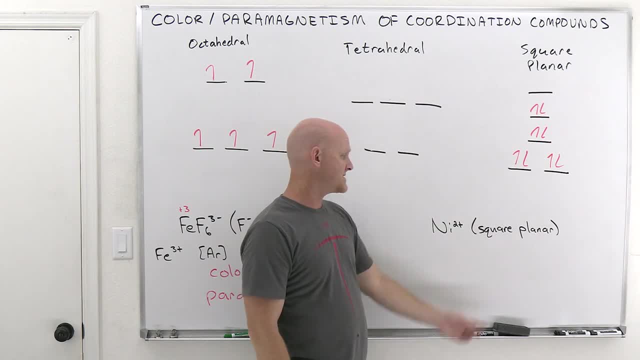 in a square planar complex And in this case, if they tell you it's square planar, you should automatically know that it's going to be d8.. But if we figure that out, so nickel is usually argon 4s2- 3d8.. 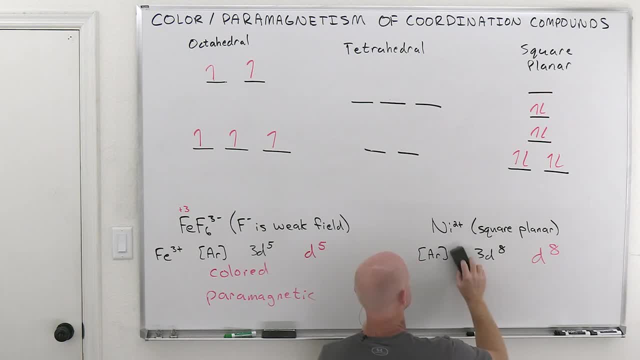 And then we lose two electrons to become nickel 2 plus, and lose the 4s's And yeah, it's just argon 3d8.. So, but square planar has to be a d8. And it has to fill in, just like this. 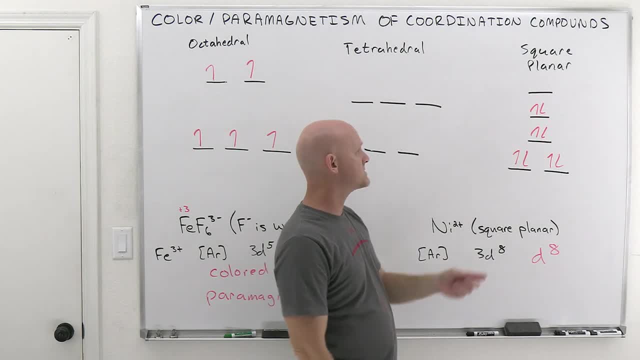 for a square planar, And so, yes, you're going to expect every square planar complex to be colored, because you have electrons down here and you have an empty spot right up here. it could go to So, but also if you fill in eight electrons. 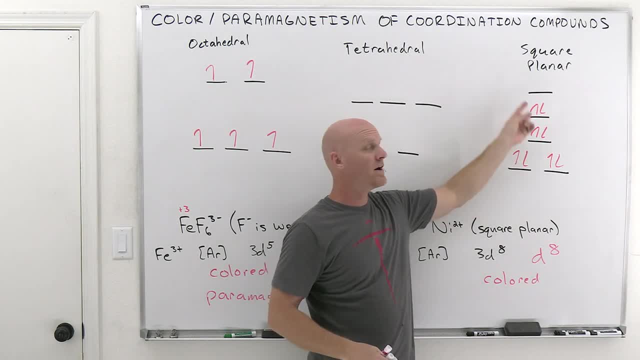 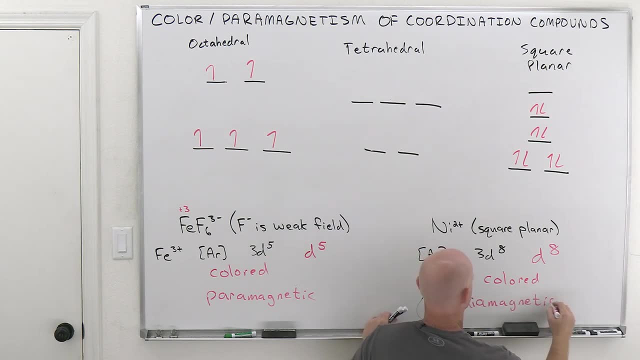 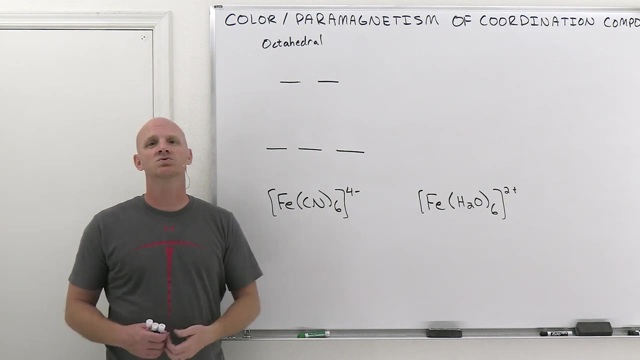 on the square planar splitting pattern. they're all going to get paired up every time, And so this guy's going to be diamagnetic, All right. So the last question we're going to deal with is which of these two lovely complex is more likely to absorb blue light. 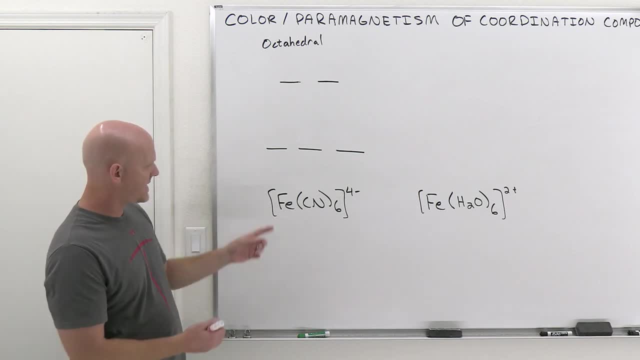 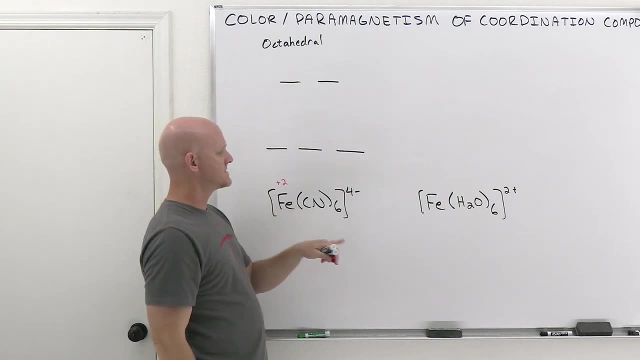 All right. So if we take a look here- in this case with FeCn6 4-, you got to realize that you've got iron in the plus two oxidation state. So each of the cyanides are minus one, And so iron must be plus two. 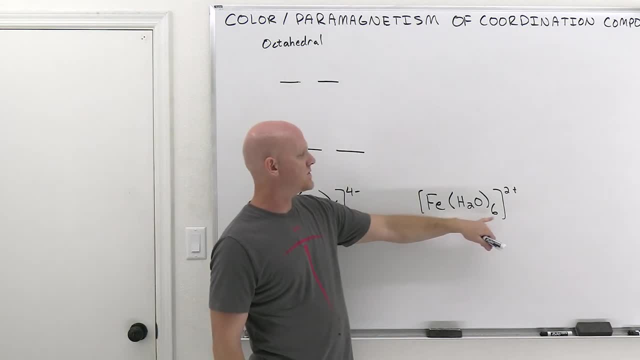 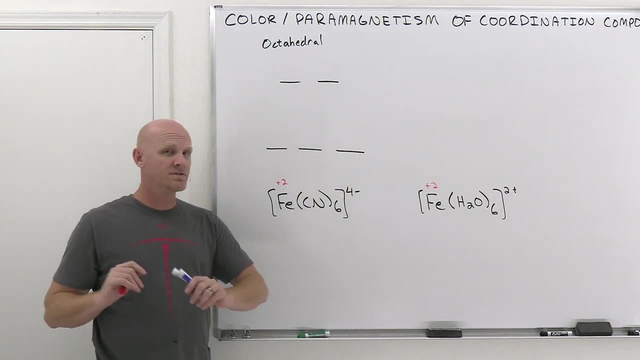 to get an overall minus four charge. And then FeH2O6, the aquas are neutral. So if it's going to be plus two, it's all due to the iron. He's plus two. So we're dealing with Fe2 plus in both cases. 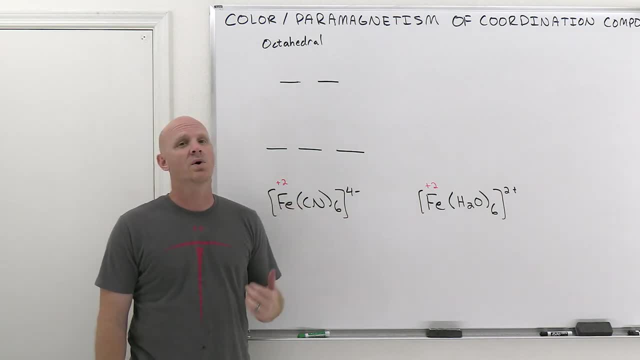 And so, in this case, the only way you can answer this question is if you are familiar with the spectrochemical series, And in this case it's on the handout. I'm expecting you to look at this. I would just not ask this blindly. 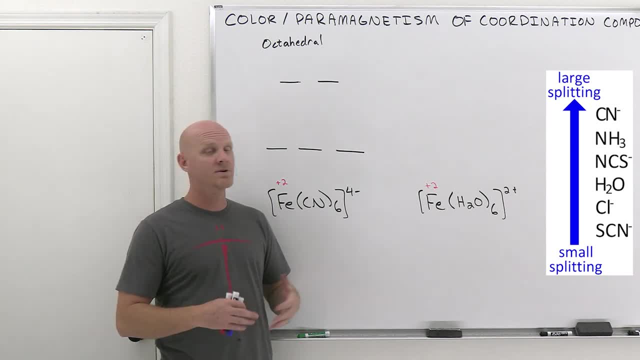 I would provide you with a brief spectrochemical series before asking you this question, And so the thing you got to look at here is that cyanide is the highest ligand on the brief spectrochemical series I give you, which means it's going to result. 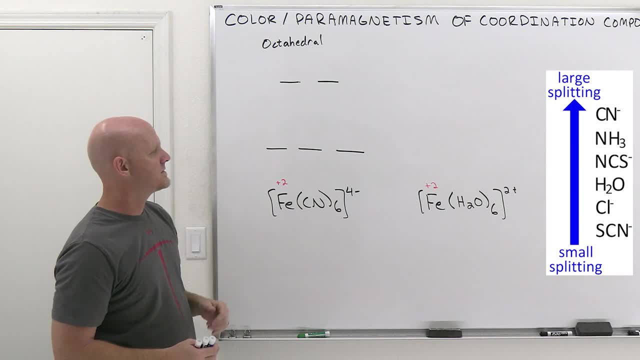 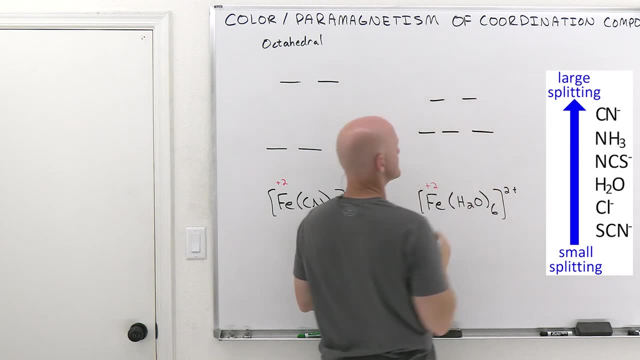 in the largest splitting crystal field, splitting energy here between those, Whereas water is lower, And so this crystal field splitting energy associated with this complex is going to be smaller. Now, in this case, I never said if it's high spin or low spin. 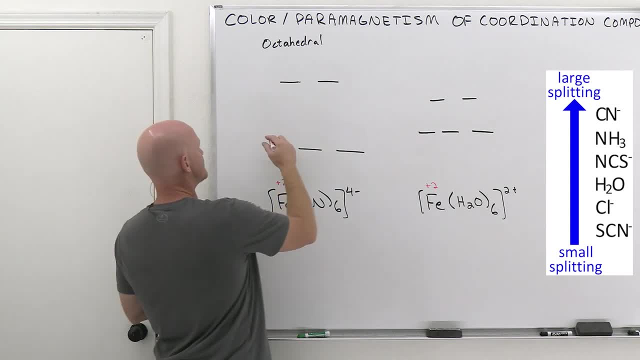 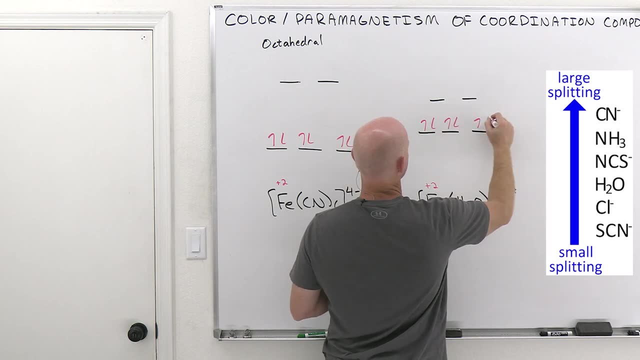 So because I'm largely not going to care. So if we just fill this in, say one, two, three, four, five six, One, two, three, four, five six, So whether I fill them both in low spin. 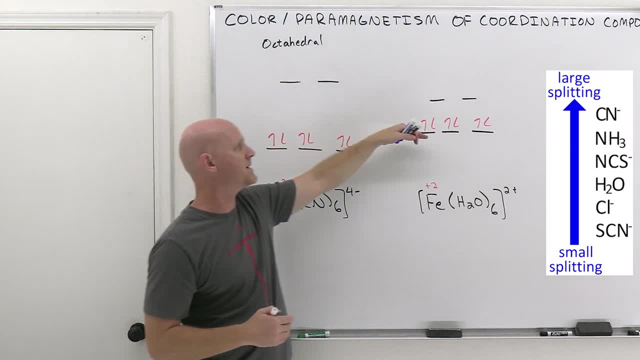 so, well then, the energy that's going to get absorbed is again the crystal field splitting energy, the energy of the light that's going to get absorbed, It's going to correspond to that energy in either case. So, and had I filled, say this one: 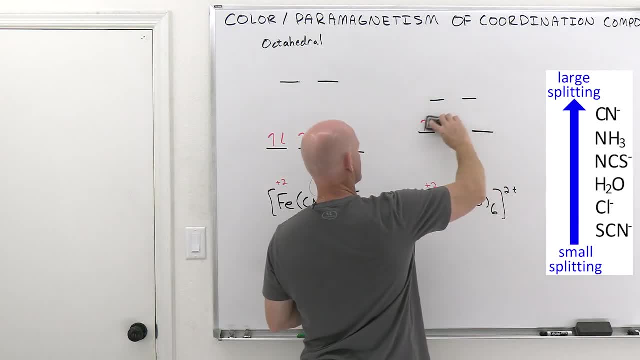 and I'm like: well, maybe this one's high spin because it's a smaller crystal field splitting energy. Maybe that's true And it's still not going to matter, because whether I go one, two, three, four, five, six, 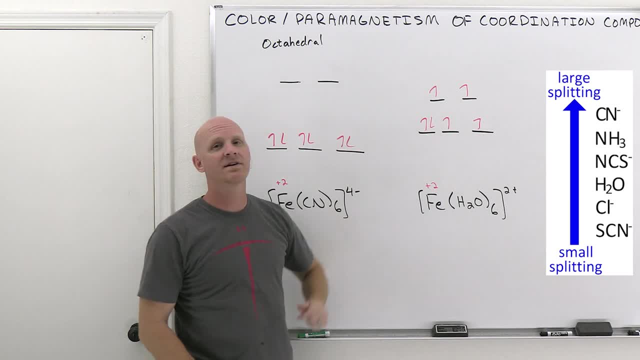 So the energy of the light that's going to get absorbed is still going to correspond to exactly the same crystal field splitting energy, And so whether these are low spin or high spin in this example does not matter. It's totally irrelevant. So the big thing. 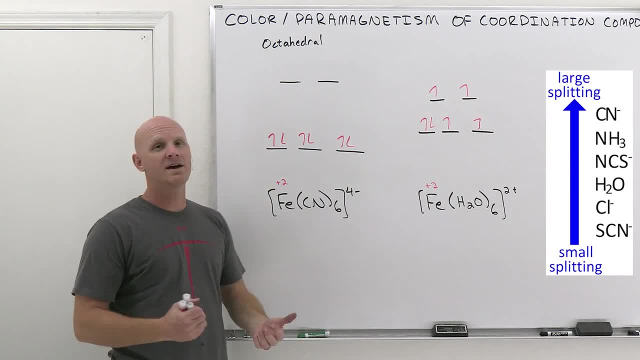 you're supposed to take away is if one of these is going to absorb blue light. well, blue again is at the high end of the visible light spectrum, So I want to pick the largest crystal field splitting energy, The energy of the light absorbs. 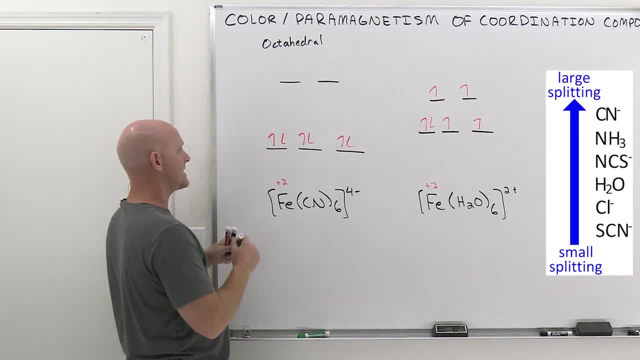 corresponds to that crystal field splitting energy. So, and in that case, therefore, I would pick FeCN6, four minus, to be closer to the blue end of the spectrum for the light absorbed. I'd expect FeH206 to be closer to the red end of the spectrum. 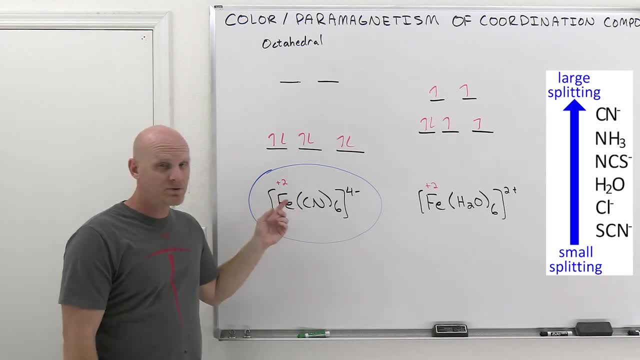 for the light being absorbed. Again, I don't know that this is actually going to be blue light being absorbed, And I don't know that this is actually going to be red light being absorbed. It's just this one's closer to being at the blue end. 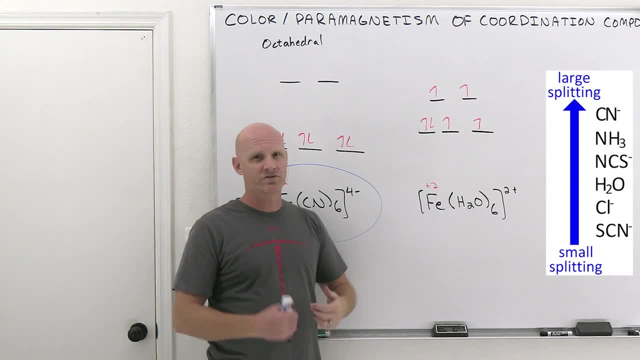 of the spectrum, And this one should be closer to being at the red end of the spectrum. And so oftentimes we just define the visible spectrum by its extremes: the blue end at the higher energy and the red end at the lower energy, that sort of thing. 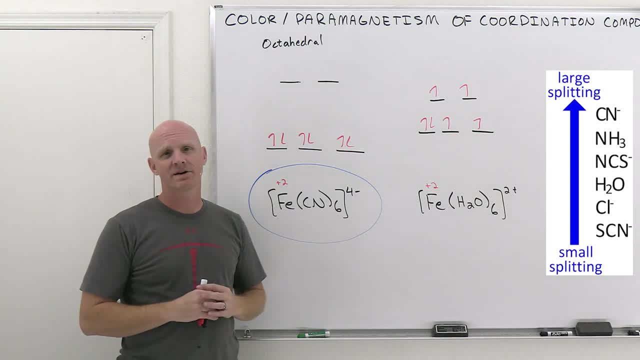 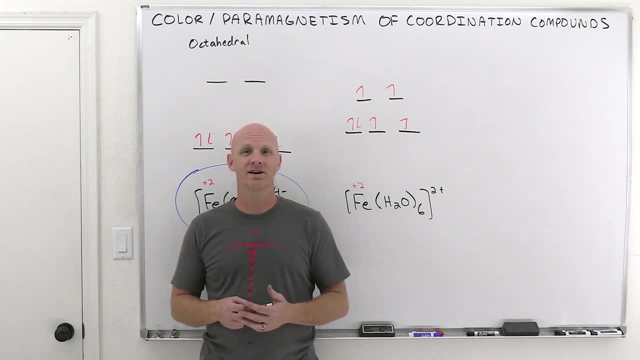 Cool, And that's exactly how that works with using that spectrochemical series. Now, if you found this lesson helpful, a like and a comment let me know are pretty much the best things you can do to support the channel. There's another chapter. 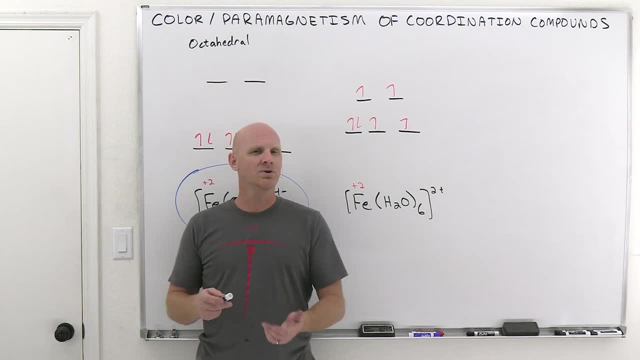 left in this playlist. It's going to be an introduction to organic chemistry And not all of you are going to get there. So a lot of classes get to the end of the semester and they just don't have time, And some just even preemptively. 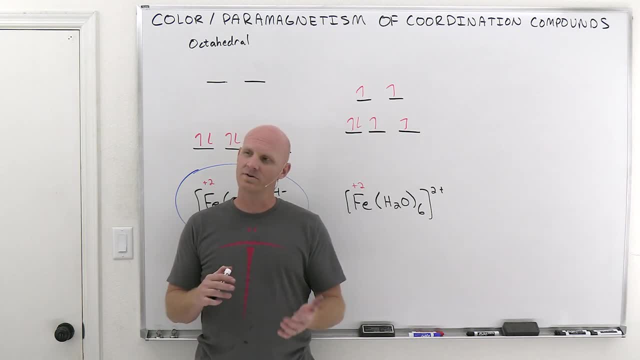 cut it off before we even get there. They don't even plan to cover it, But for some of you that are going to include that chapter, I've covered it next week. So if you want to be notified, still subscribe to the channel. 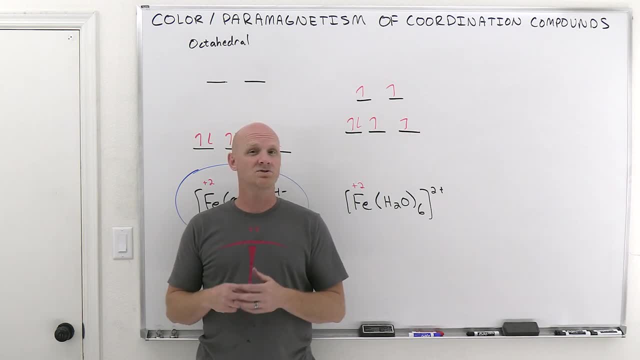 and hit that bell notification, But I'm not going to wait too long before getting going on my next playlist. So if you have again a choice between biochemistry, redoing physics or doing a freshman bio course, I'll take your vote. 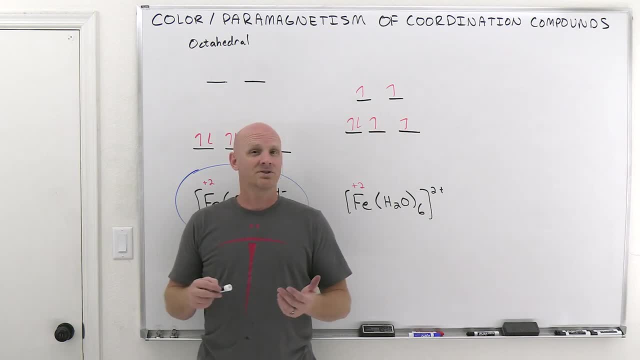 quite seriously- I'm not just trying to get comments here- And if you're studying for your final exams, take a look at my General Chemistry Master Course. It includes final exam, rapid reviews, practice final exams. if you're trying to do things quickly,